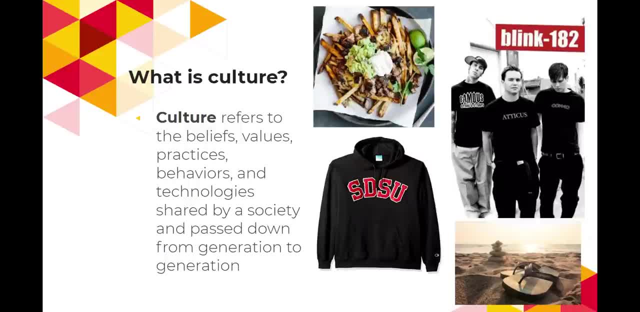 that we see where I'm from in San Diego. alright, Carne asada fries is a staple of San Diego Mexican-American cuisine. In fact, I'm going to get some of that here pretty soon. Hooded sweatshirts, flip-flops, the music we listen to. 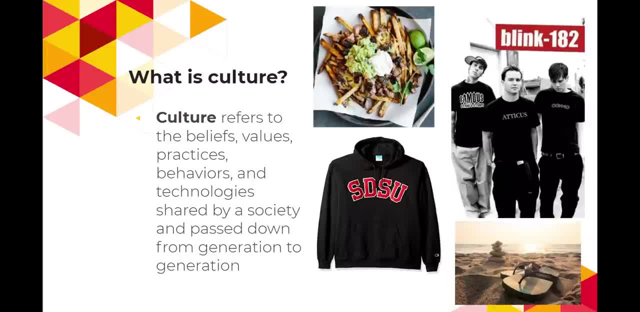 one of my favorite bands, Blink-182, all of that are. all of those are examples of material culture, alright, And it's a lot different from non-material culture, which is a little it's a little bit tougher to see, but we still experience it. 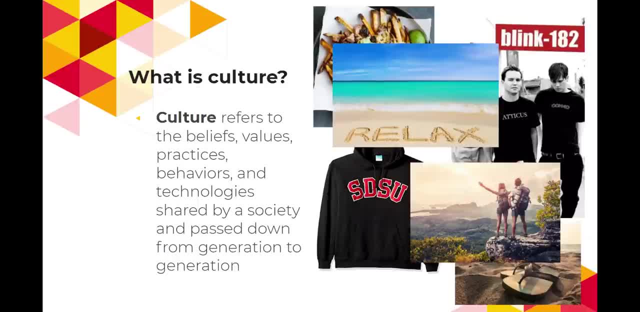 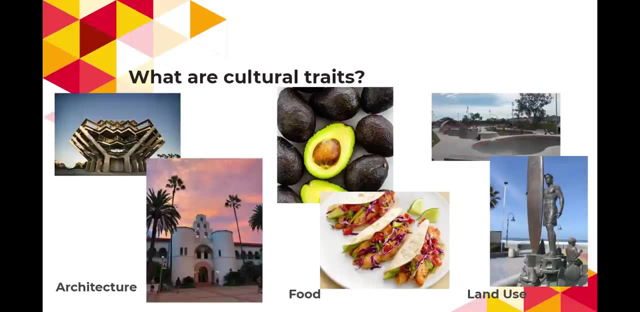 And those are the values we have, or the beliefs we have, Things like relaxing by the beach or being adventurous and wanting to spend time in the outdoors. Those are all values that are kind of unique to San Diego culture. okay, Now let's get into some cultural traits. 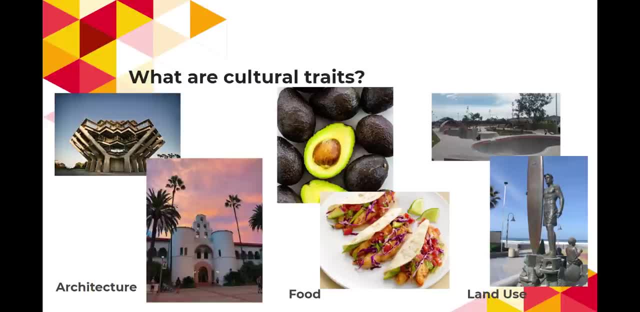 And cultural traits could be anything. It could be architecture, it could be food, it could be land use the clothes you wear, the television you watch, the music you listen to. These are just a few examples of cultural traits that are kind of obvious. 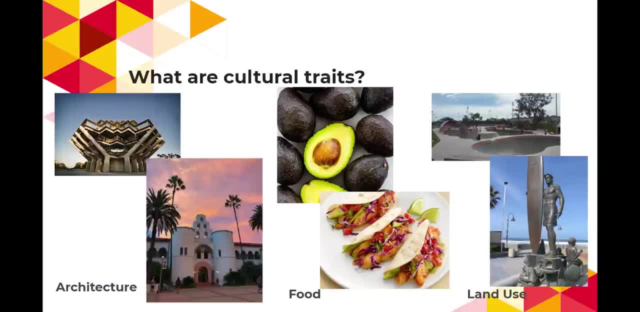 and ones that you can see in my community of San Diego, Whether it's those college campuses that you see down there on the lower left, the Mexican food that you see in the center, or even the way we use our land, Whether we have skate parks in different parts of San Diego. 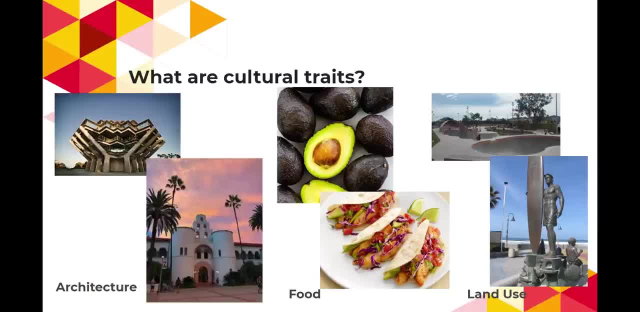 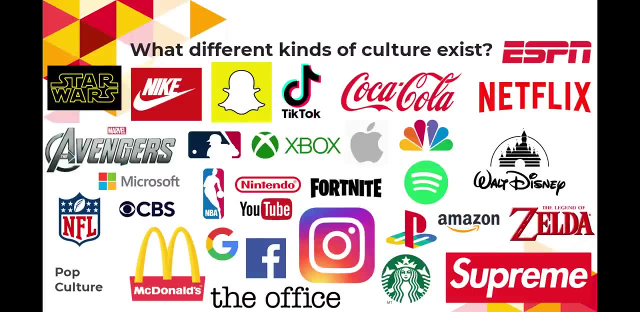 or monuments to surfing, like we have in Imperial Beach. alright, Now, all of these cultural traits um manifest themselves in two different kinds of cultures that human geographers are concerned about, And the one that's probably most familiar to you is pop culture, right? 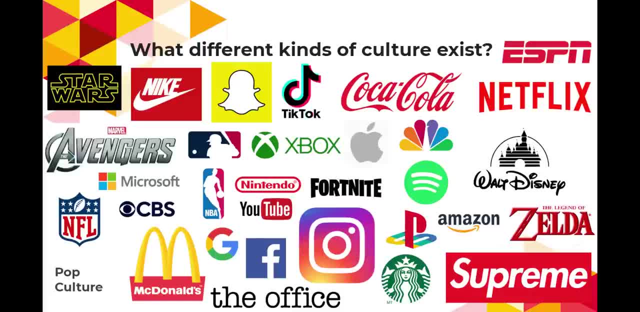 You probably recognize nearly all of these brands and logos that you see here on the screen because they're everywhere. They're very prevalent, They're a part of pop culture. Lots of people in the United States and around the world today enjoy eating McDonald's. 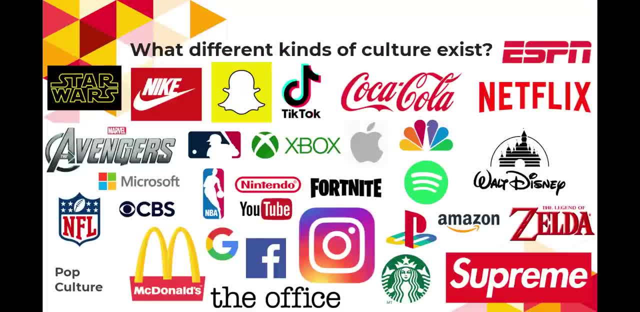 They enjoy watching Netflix, They enjoy drinking Coca-Cola, They enjoy watching Star Wars or wearing Nike. These are the brands, the technologies, the shows, the types of music, the sports that are very common, very popular and very prevalent throughout our society. 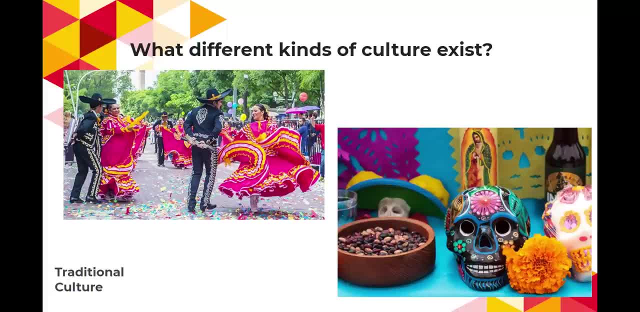 And this is a lot different from traditional culture. Traditional culture or local culture, or sometimes it's even called folk culture. um, they all relate back to, uh, specific places and they're kind of slowly dying out as a result of the prevalence of pop culture. 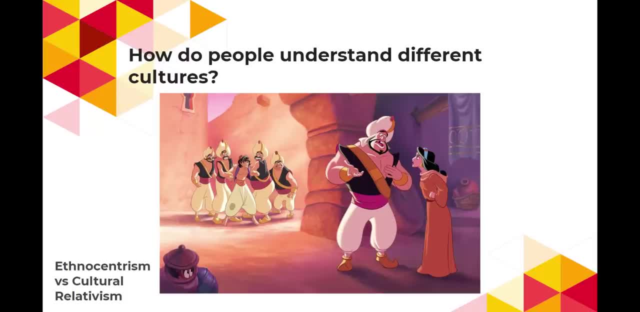 Okay, Now, how do people understand different cultures? There's basically two schools of thought here, uh, one that we call ethnocentrism and the other that we call cultural relativism. cultural relativism- And you see, on this screen, 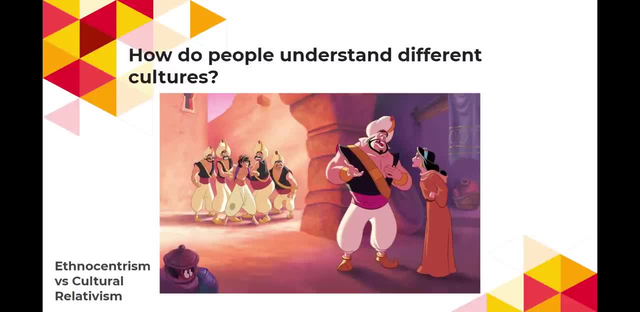 I have an image from from, in my opinion, a pretty good Disney movie, uh, one that you're probably familiar with, in Aladdin. All right Now, unfortunately, from our 21st century perspective, Aladdin has a very ethnocentric view of the world. 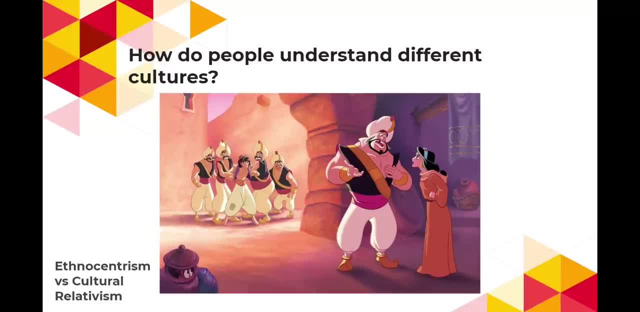 And even in this image you can kind of see it where all of the bad guys in this image have have a beard right. Um, and you'll probably remember from the movie that two of the only characters who have American accents are the good guys in Aladdin and Jasmine. 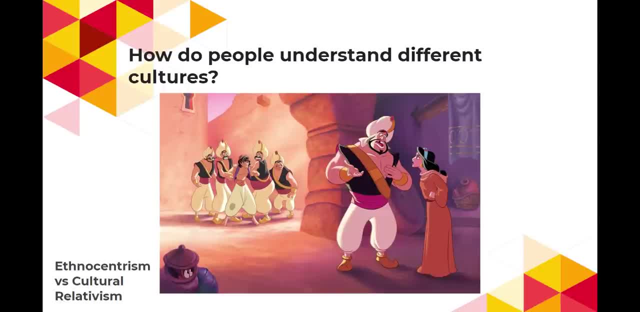 right, Um, everybody else that either has a Middle Eastern accent or a British accent, and what the filmmakers did. And remember, this is the movie that was made in the nineties, So you know, this type of idea wasn't as. 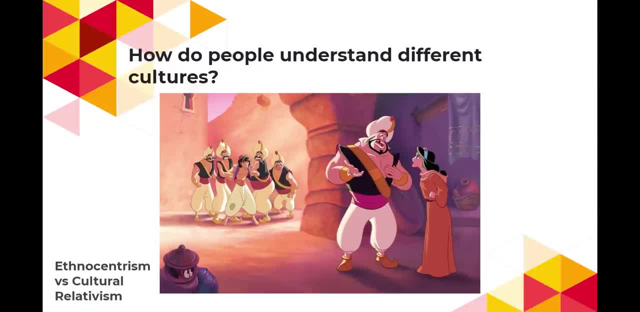 uh, influential back then. but what the filmmakers ended up doing is they projected American culture onto this Middle East setting and they made the. they gave the heroes very prototypical American traits, like an American accent, like a clean, shaven face. Um, 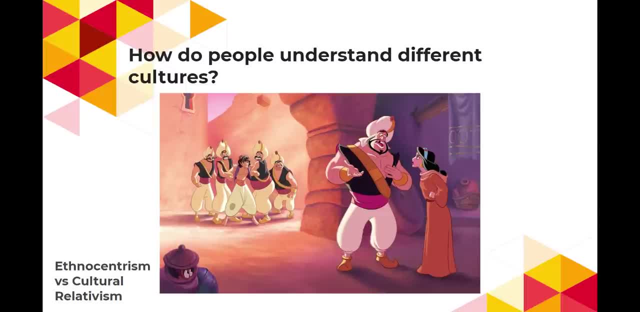 even Aladdin has lighter skin than the bad guy like Jafar Um. so all of those are examples of ethnocentrism, and Aladdin gets a lot of criticism from our 21st century perspective because of that. All right. A better way of interacting with different cultures is to understand them from where they're coming from. 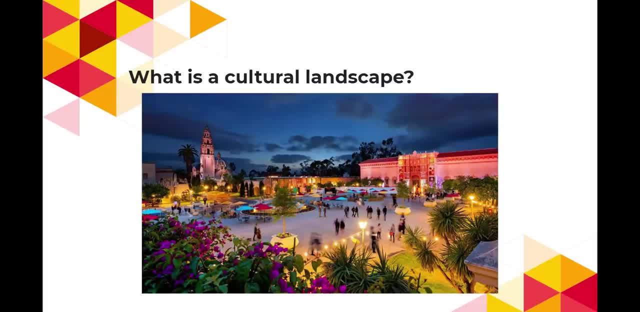 And we call that school of thought cultural relativism. All right, let's move on to cultural landscapes. So if you look outside, if you were to go outside your house or to go walk down the street, everywhere around you you can see the built environment or the cultural landscape. 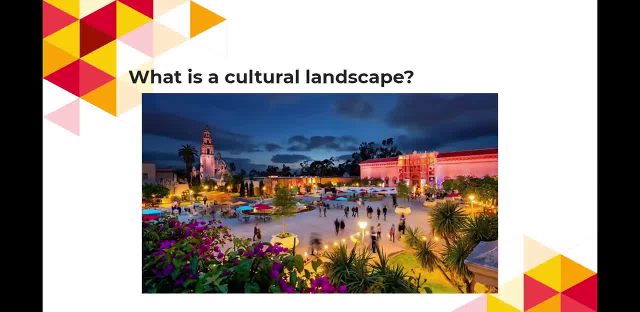 right, This is different from a physical or a natural landscape, which is going to be, you know, the surface of the earth that has been relatively untouched By humans. So, if you're looking at a mountain or a lake or a river, 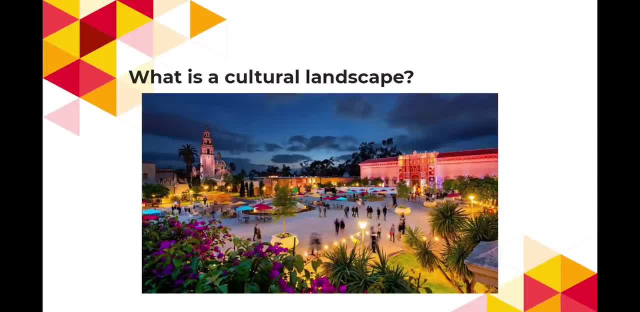 that's the physical landscape or the natural landscape, And that's a little bit different than the cultural landscape. The cultural landscape is the built environment. It's what the humans have done to the surface of the earth, And what we did in my class is we had some practice reading cultural landscapes. 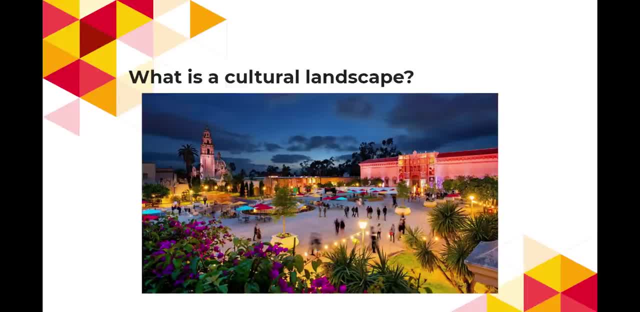 And what you see in the image. here is a picture of Balboa Park in downtown San Diego, And there's a lot of things you can pick out of this image that tell us about the society of San Diego, What San Diegans have felt to be important over time. 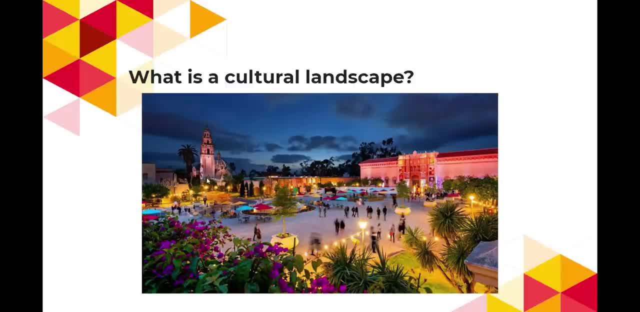 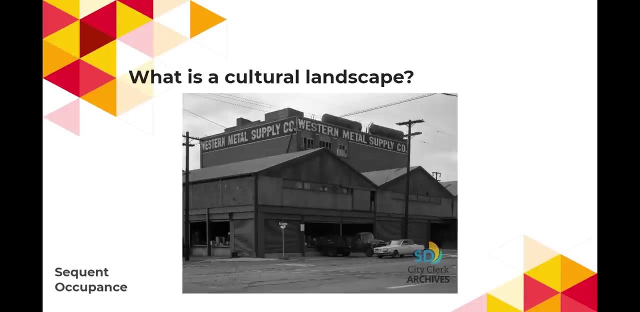 whether it's the the traditional Spanish architecture of the California tower back here in the distance or also here in this museum. you see the traditional Spanish plaza right there as well. There's a lot of Spanish influence in a place like Balboa Park, and San Diegans throughout history have felt that that's pretty important for us to preserve. 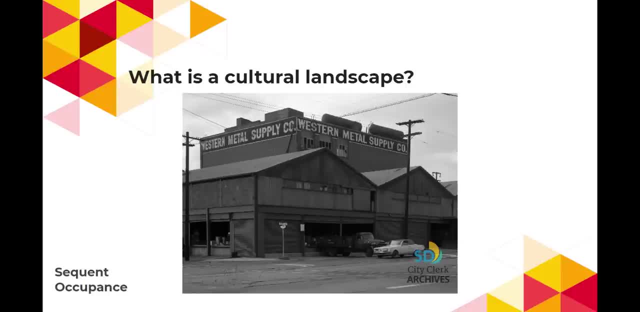 All right. Another key aspect of the cultural landscape is this idea called sequent occupants. Sequel occupants is essentially what humans have done to the landscape through time and as different cultures have kind of cycled through the landscape. So you see this historical photo right here of the Western Metal Supply Company building. 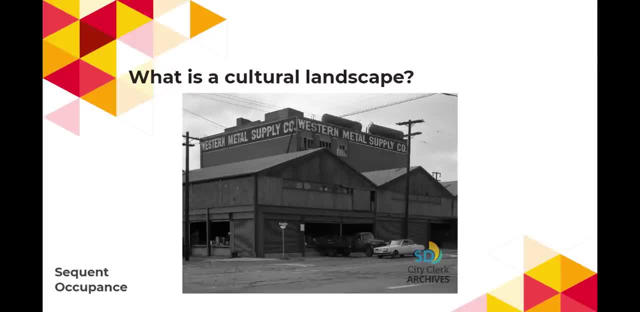 All right, If you're a fan of the Padres, like I am, then this building probably seems a little bit familiar to you, because it's not used as a factory anymore, as a warehouse anymore, But now it's the left field of Thalpole, at Petco Park. 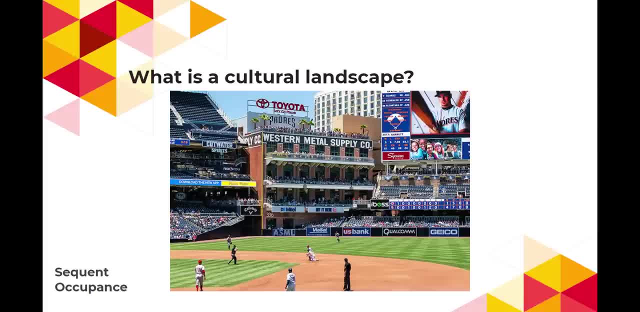 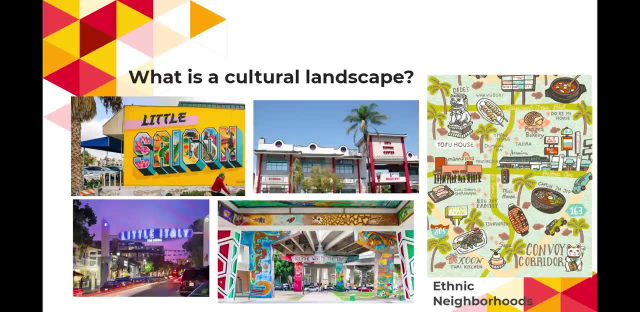 So different cultures and different societies have used this building in different ways, whether it was previously as a warehouse or now as a pretty cool feature in a baseball field. All right. Another key aspect of cultural landscapes are called ethnic neighborhoods. All right, And we have a lot of them in my hometown of San Diego. 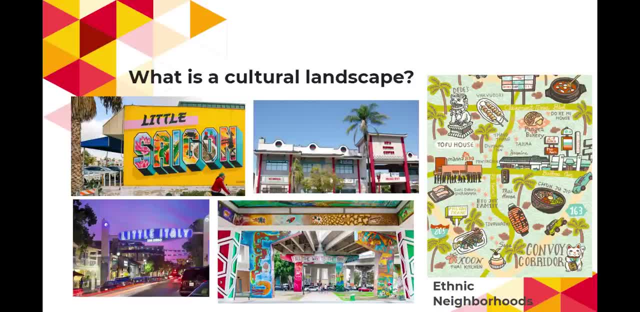 whether it's Little Saigon and the City Heights neighborhood, Little Italy, Barrio, Logan and Chicano Park down here, or the Convo neighborhood in the northern part of San Diego, All of those ethnic neighborhoods celebrate different types of cuisines, different traditions from various places around the world. 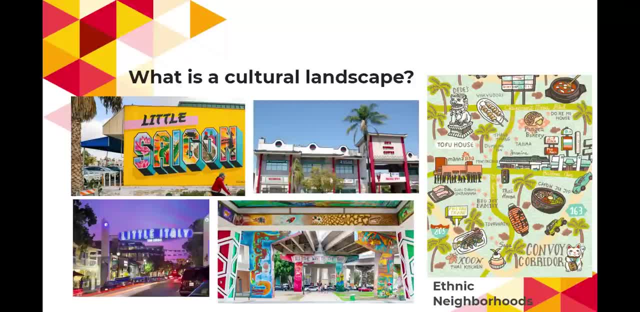 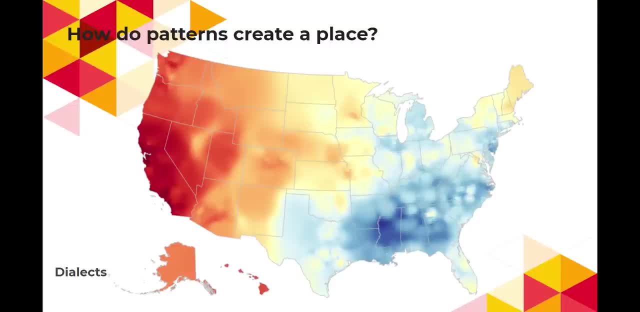 And they give San Diego a bit of a unique character and also like a unique neighborhood and unique destination for us locals to go to. All right, Let's get into patterns, cultural patterns, and how these cultural patterns create places. My class will probably. 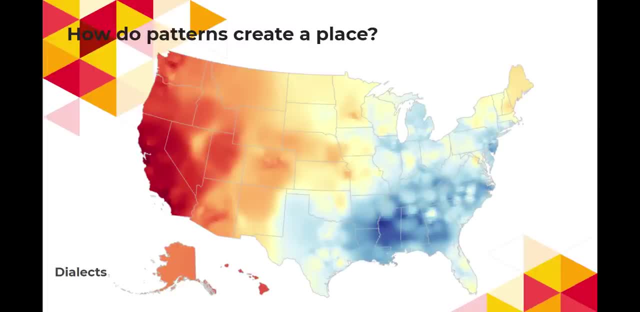 Remember that we took the New York Times dialect quiz and I actually took the quiz again in the lead up to this video And I got this map and you'll see that California is the darkest right over here, meaning that the dialect that I came up with on the quiz was most shared in this area of the United States. 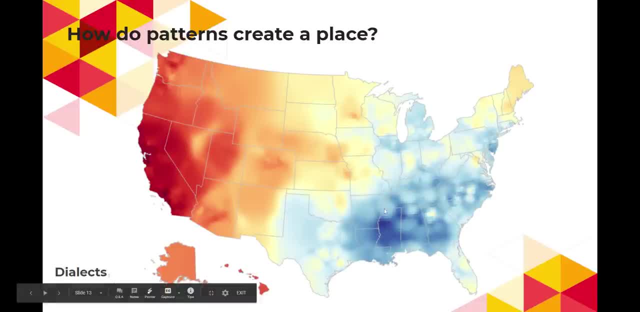 It's a lot different than the deep south. right in the deep south, They speak a very different type of English than I do, So you'll see that this region of the country is a deeper shade of blue. Okay, But dialects play a large role in creating a place. 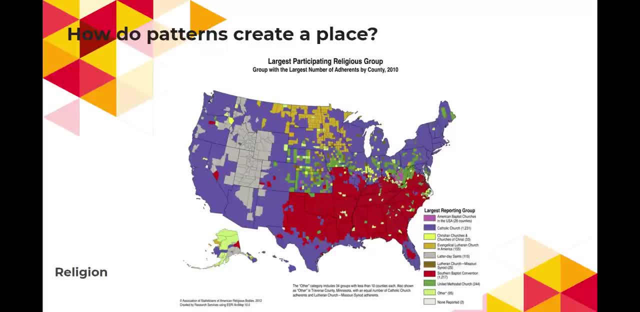 All right. Another key aspect is religion, or majority religion, And this map is unique because it shows us the largest religion within a certain area- Okay, Whether it's Catholics are all in the purple areas, or Latter-day Saints in this area and primarily Utah and the surrounding states. 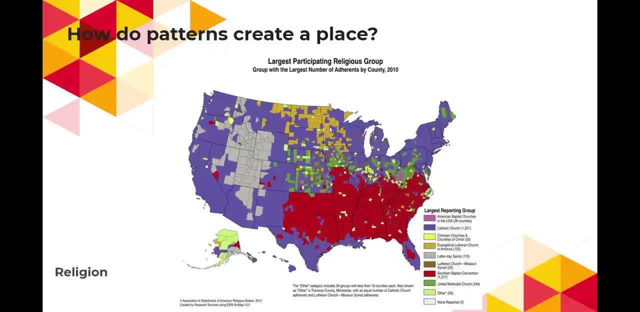 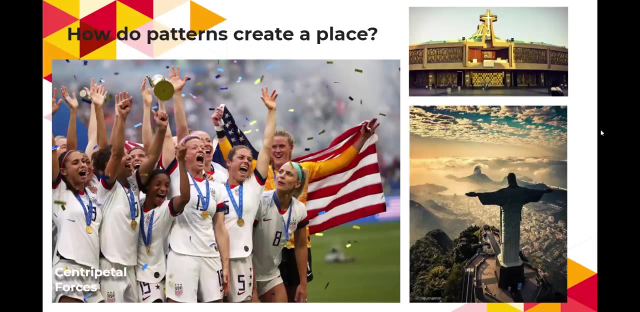 Lutherans up in the northern part of North Dakota, Minnesota, South Dakota into Wisconsin a little bit, or Southern Baptist throughout much of the southern United States, all the way as far west as Texas and as far northeast as into Virginia and North Carolina. All right. 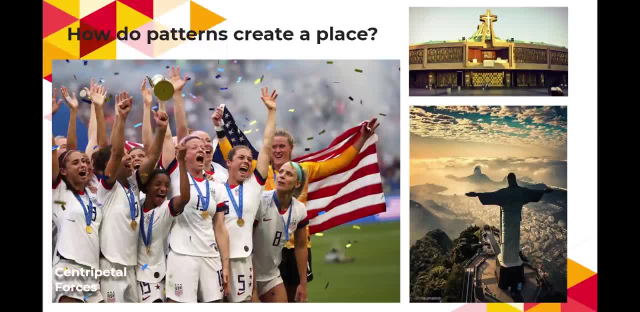 Let's talk about centripetal forces. So centripetal forces are these forces that are going to connect people or have people feel a stronger attachment to the place in which they live? All right, Historically, language and religion have played a very 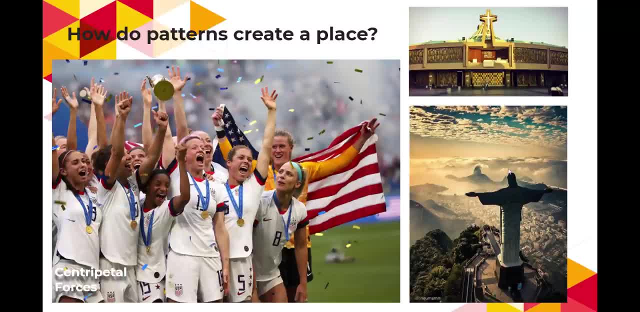 very large role in that. And you see that because in Latin America Christianity is access Since triple force, despite the fact that Christianity started- and an entirely different continent a long time ago, before the Europeans ever came to the Western hemisphere. So you see that, either in Mexico City, at the Basilica of Our Lady of water Lupe, or in Rio de Janeiro, where Christ 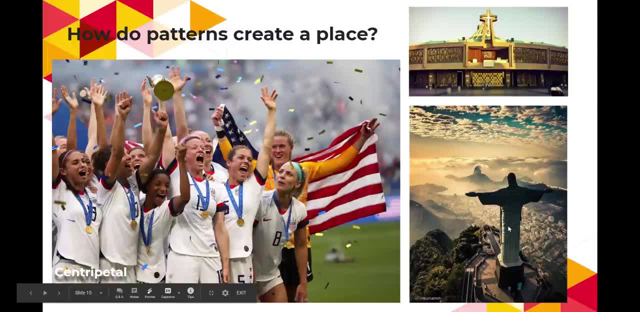 the Redeemer sits atop this mountain overlooking the city. But it's not always language and religion that it's going to play a centripetal force. even sports can play a role in that. so you see here, um, the united states women's soccer team. this is right after they won the women's world cup in 2019. and um, i went to petco. 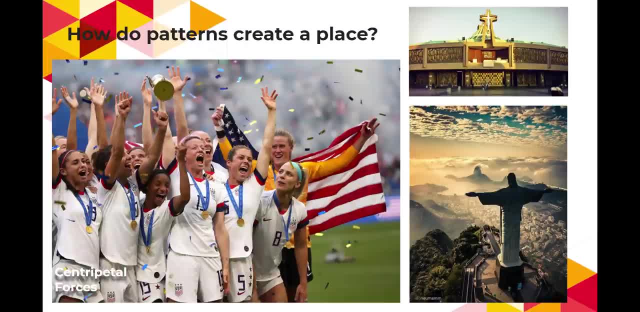 park to go watch that match, uh, with my son and with my wife, and everybody was going crazy cheering for the united states, and, uh, you felt this palpable american pride in that moment and it really served to bring people together, to rally together around. you know, just something as as kind of 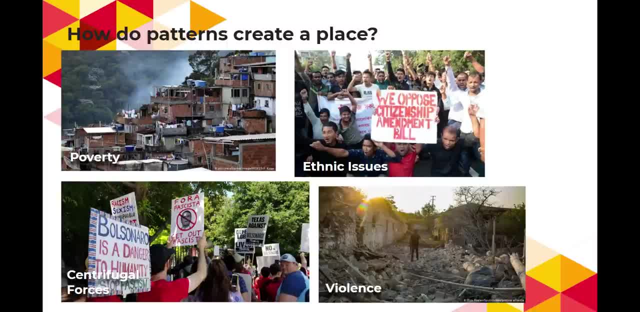 inconsequential as a as a winning soccer team, all right um. centrifugal forces, on the other hand, are forces that create divisions amongst people, and there's lots of different causes of central fugal forces, whether it's poverty, ethnic issues or violence, like you see here in this image of. 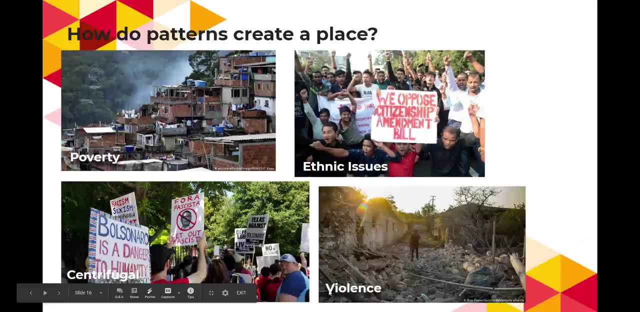 mcgoronokarabak, um, in the central asian region, um, those are going to be forces that create divisions between people and make it so that people don't see quite eye to eye, and this could have a negative effect on people's lives, and i think that's going to be a big issue for me in my 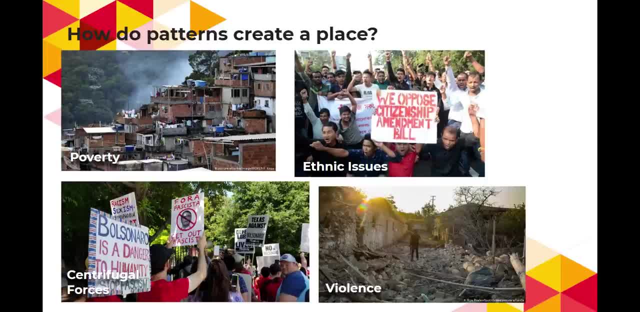 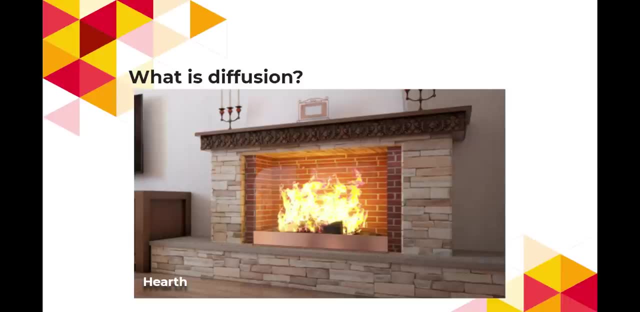 have a lot of different effects, whether it's um independence movements or socialized social isolation, um or other effects that we'll get into, uh, in the next video on unit four. all right, let's talk about diffusion for a little bit. um, when we're talking about diffusion, we got to talk. 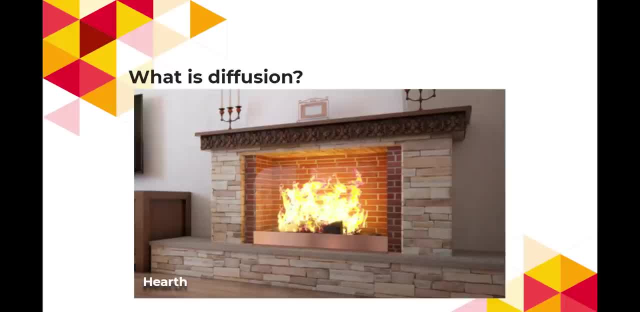 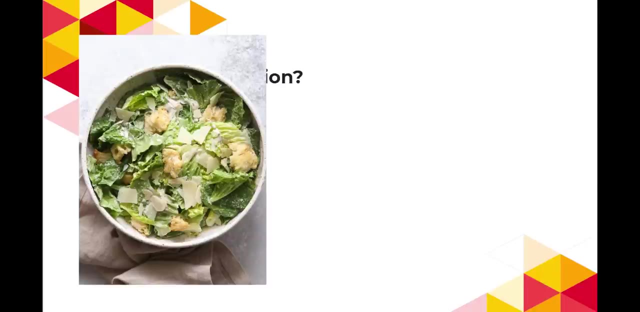 about hearts. hearts are where things came from. so think about like a fireplace. the fireplace begins in the hearth right, that's where the fire starts, and then that idea diffuses out to other places. all right, one example: i like to use the caesar salad, a staple of some of my very favorite. 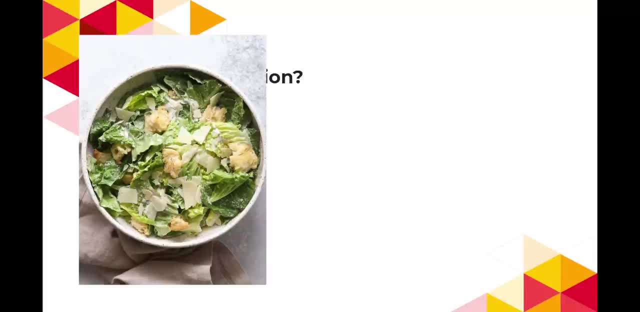 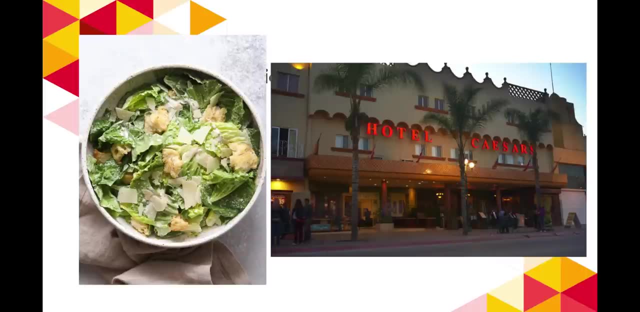 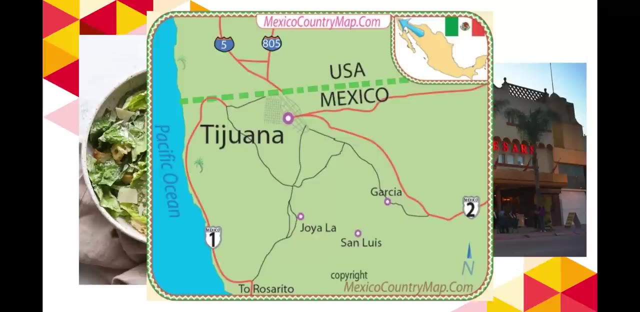 italian restaurants, um, and you would think that it had its hearth, um, probably in italy, right? well, in reality, the caesar salad was started the hotel caesar in tijuana, california, mexico. all right, a little surprising probably for some of you, but the hearth of the caesar salad was actually not. 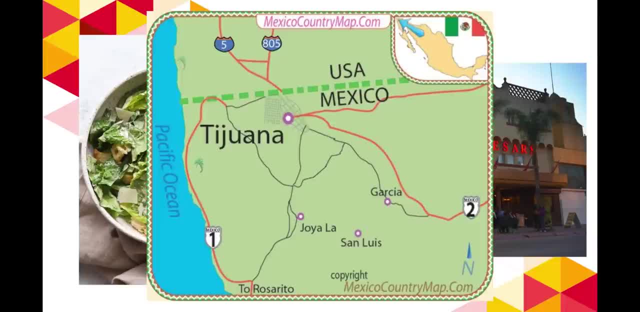 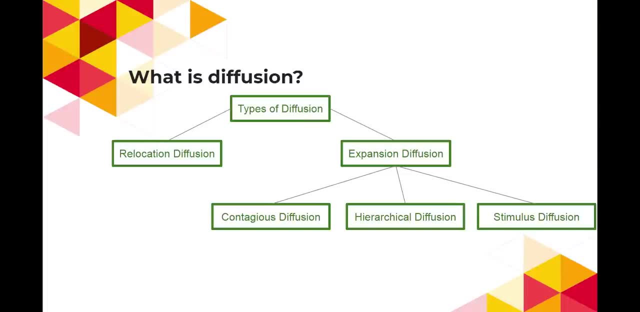 just not too far south from here, just about 15 miles from where i am right now, um just south of the border in tijuana. okay, yeah, caesar salads are our mexican food. so, uh, types of diffusion. we have two main types. we have relocation diffusion and expansion diffusion, and we'll talk. 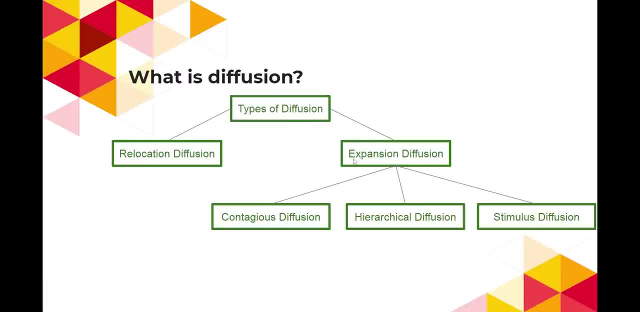 about relocation diffusion in a second um, but it's important for you to know that. then there's three different subtypes of expansion diffusion as well: uh called contagious diffusion, hierarchical diffusion and stimulus diffusion, and uh, we'll talk about each of those in just a moment. all right, but 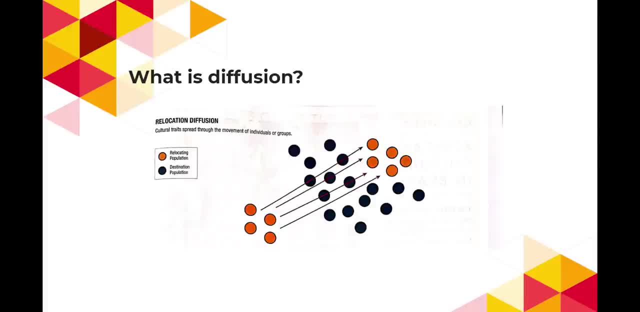 first let's do relocation diffusion. this should be the easiest type of diffusion for you to kind of visualize in your mind, because this is when either someone or something is moving from one place to another. all right, so let's think about that caesar salad again. right, that caesar's, that idea, the caesar. 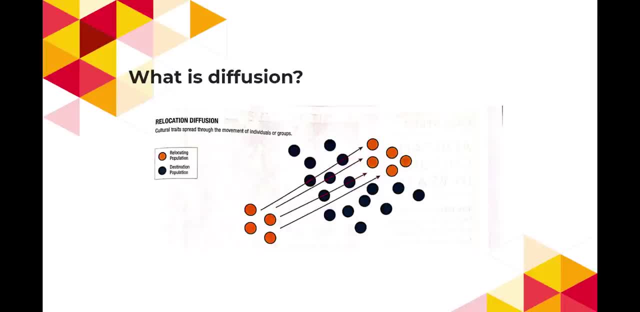 salad probably initially diffused pretty rapidly throughout tijuana and, i'm assuming, san diego as well, through relocation diffusion. all right, whether somebody, just you know, heard about this awesome salad and they wanted to take that to another part of tijuana, or they wanted to take 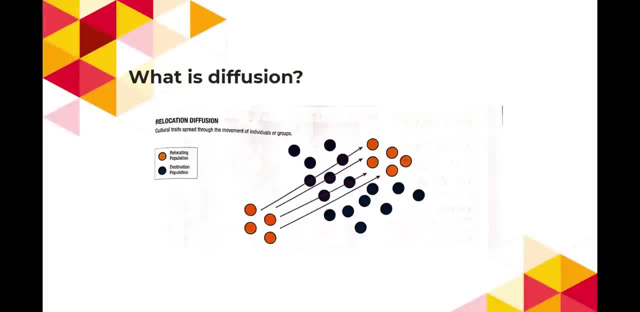 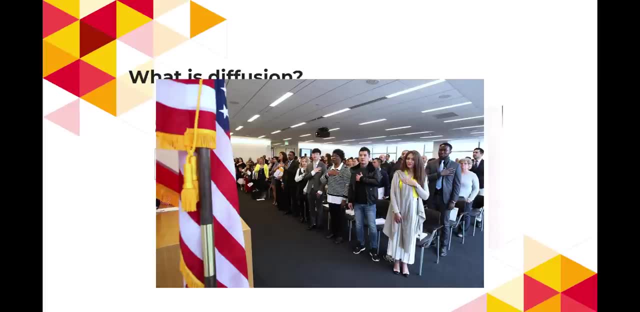 it home, or or they told somebody in san diego about it. that idea of the caesar salad just essentially got up and moved from one place to another. okay, another type of relocation diffusion? uh, that you can, that we see every um all the time here in the united states. are people moving here? 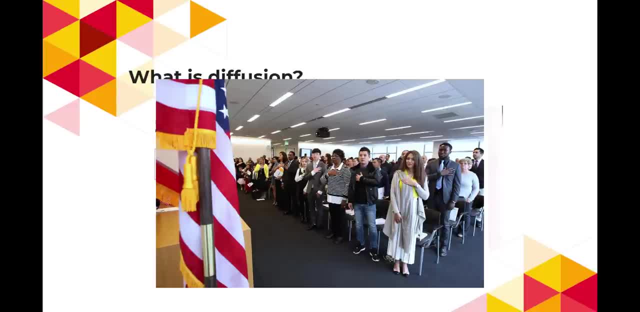 the united states and becoming american citizens. all right, you see here an image of of a lot of new americans, right? americans who are taking um the pledge of citizenship to be a member of this country. um, and they all relocated, right, they relocated from wherever their home. 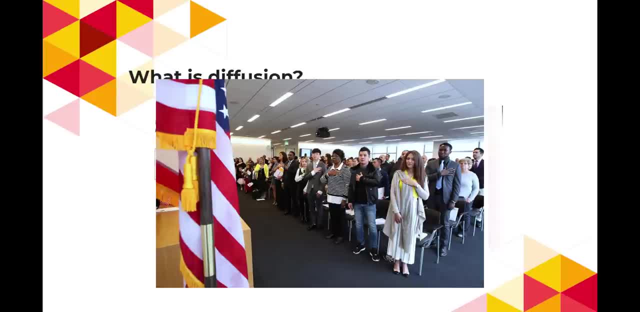 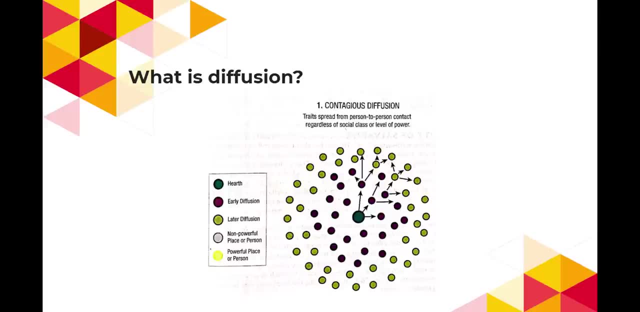 country was, and now they are becoming an american here in the united states. all right. next let's talk about contagious diffusion. so contagious diffusion diffuses from person to person, right? it spreads regardless of power, it spreads regardless of class, it spreads regardless of race or ethnicity. it just goes everywhere. right, and the 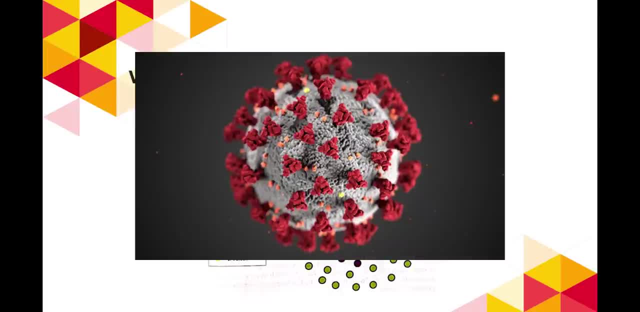 example i could give you is the thing that's on everybody's mind right now. is the coronavirus right? the coronavirus doesn't care whether you're rich or poor, whether you're male or female, whether you're black or white, whether you like the yankees or the red socks. coronavirus spreads. 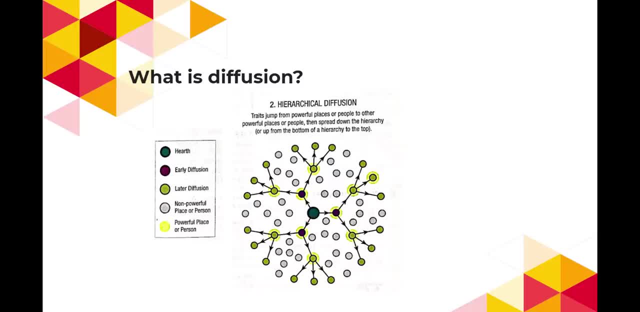 in a contagious fashion to everybody. all right, uh. hierarchical diffusion is another example, and this one. this idea spreads in like a top-down approach. okay, so essentially, somebody who is more influential or more powerful might have this idea, or they might come across this idea and they're going to use their 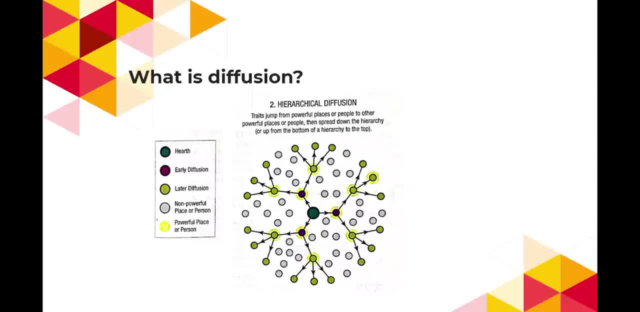 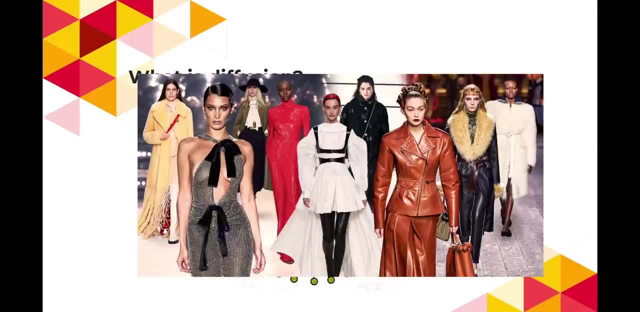 influence, to spread it to people who are relatively less powerful or influential right- and a great example of this is fashion right- somebody famous wear something on, either in a fashion show or maybe even like in a tick tock or an instagram story, and then that idea catches on. 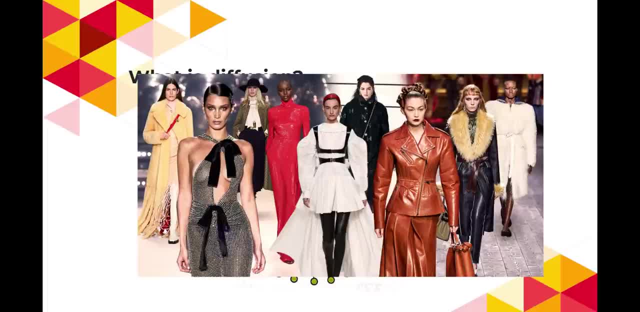 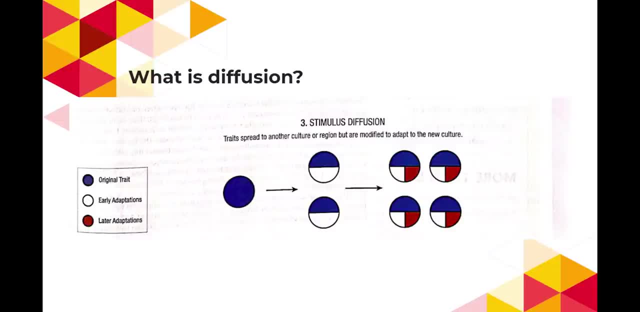 and then it diffuses downwards to people of relatively less influence, people of relatively less power. all right. next we got stimulus diffusion, and in stimulus diffusion the thing that's diffusing is changing a little bit, right. so you see, like this blue circle, it's diffusing off onto the 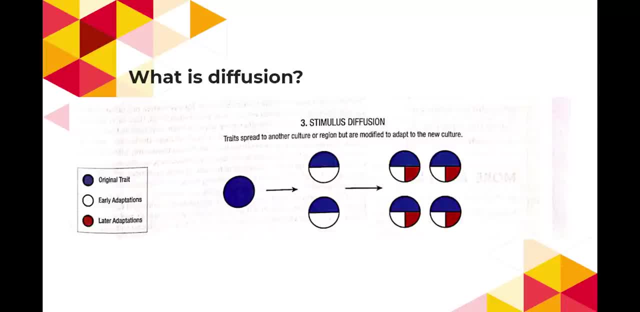 right word: part, uh, half of the screen, um, but it's not staying just completely blue. it goes from blue to blue and white and then even to blue, white and red. um, and that is because it is changing. something about the stimulus is changing. a good example of that is the maharaja map, which is a 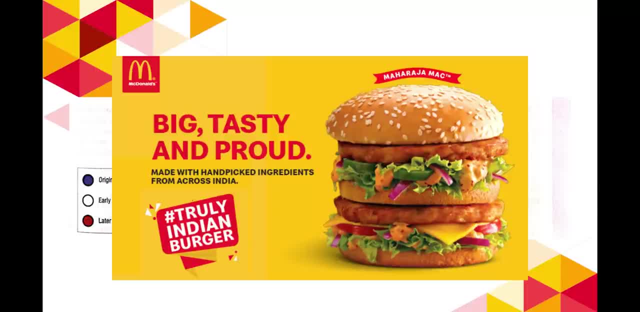 very famous one in india that made a big impact of the same thing. i'll show you that. uh right, so what it's doing is it's changing the way in which they eat at mcdonald's in india. all right, if you know anything about hinduism, you know that they don't eat cows as a part of that religion, and 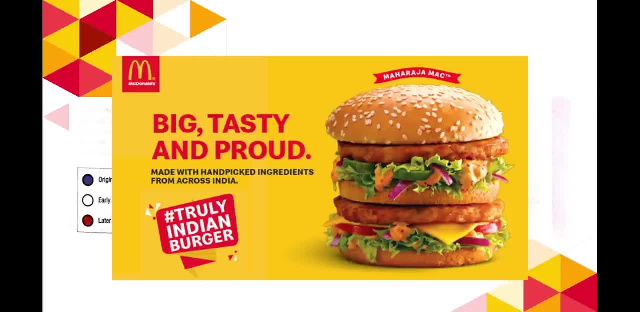 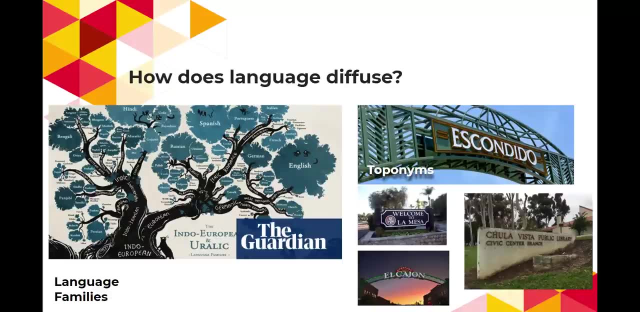 it's pretty tough um to eat a big mac if you're not going to eat cows, so they have created their own type of indian inspired cuisine that they have in mcdonald's. it's not this mcdonald's that we're used to here in the united states, but it's still mcdonald's nonetheless. 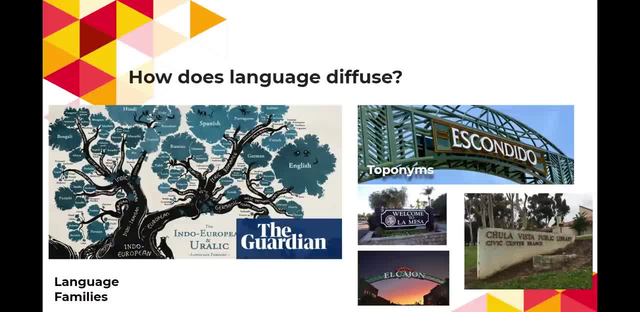 right. what you got to know to begin with is that languages come from language families, and i really love this image from the guardian of the indo-european and iraq language families. all right, so indo-european was like the original incarnation of all of these different languages. 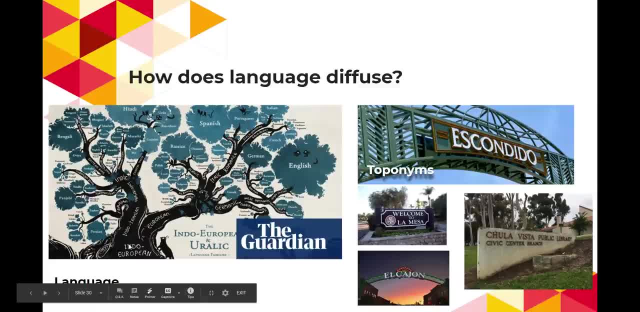 okay. and then that language, as it diffused throughout time and space, change a little bit bit by bit into different language branches, into different language groups, and then you see the languages themselves. um, which would be the leaves of the tree here in this image? all right. and then we know that there's different types of english. right, i've already? 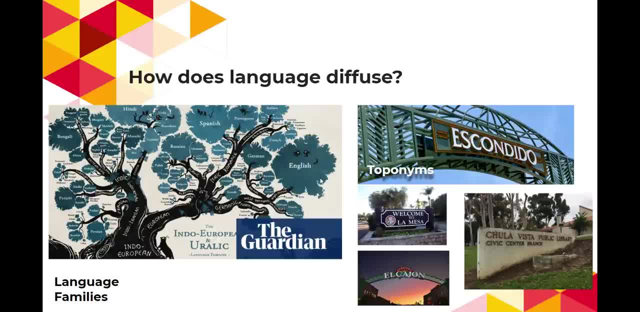 talked about how in the south they speak a different dialect of english um from what i speak here in california. so imagine all these different leaves. they probably look a little bit different. they're probably a different shape, a different size, um. all of those would be different language or different dialects, um in this example. okay, 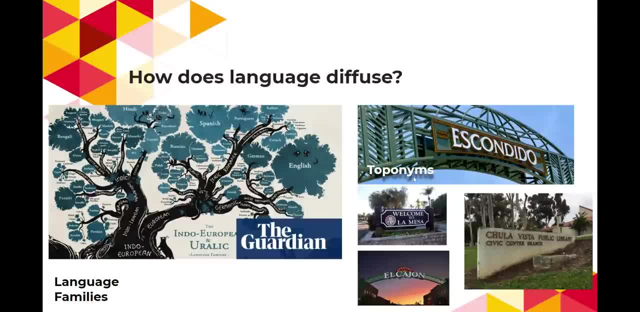 now, as a result of language diffusion, we get toponyms or place names. here in california, as we mentioned before, there's a heavy spanish and mexican influence in this neighborhood and we see that with our place names, um, here in the san diego region, where lots of our places, lots- 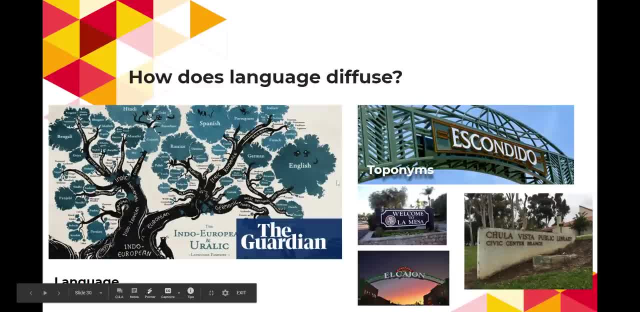 of our cities, in this example, um, use a spanish language. whether it's escondido la mesa, chula vista el cajon, those are all in spanish and we pronounce them a little differently when we're saying them, like escondido el cajon, chula vista um, but we're using the spanish language to convey those place. 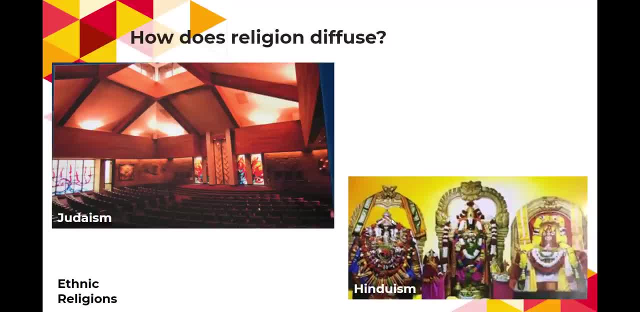 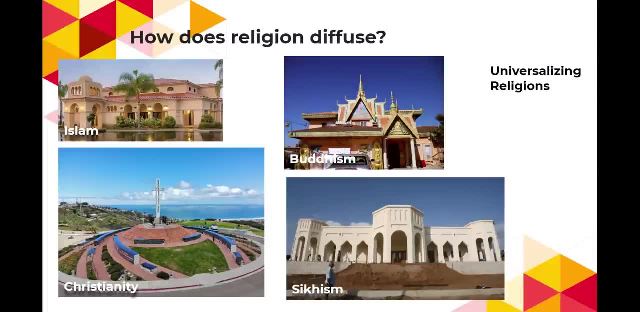 names. um, and that is because of language diffusion, all right. next, we got um religious diffusion. okay, um, skipped one. so let's go here. universalizing religions first. okay, universalizing religions. the way that i think about this is that if you are a member of a universalizing religion, you would be perfectly okay if you made everyone in the universe 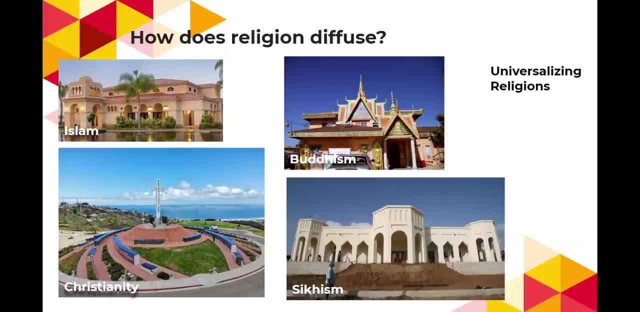 feel like that is the one true religion. you feel like this faith has something to offer to anybody, and you might even go out and try to convert other people to your faith. right, those are called universalizing religions, and there's four main examples that we would like you to know whether that's Christianity. 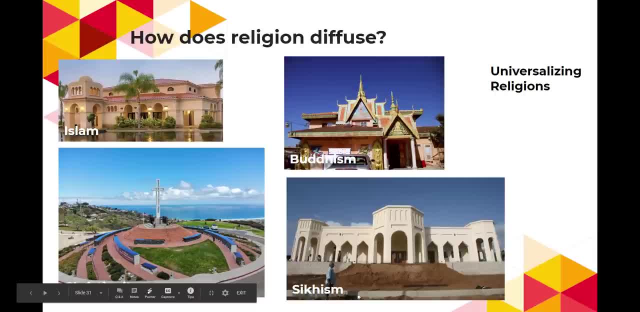 Islam, Buddhism and Sikhism. okay, and in fact you can see evidence of all four of these universalizing religions in the landscape here in San Diego, whether it's on Mount Soledad in La Jolla or this is long Islamic community center- I'm not too far away from La Jolla- or these Buddhist temples or these Sikh. I can't. 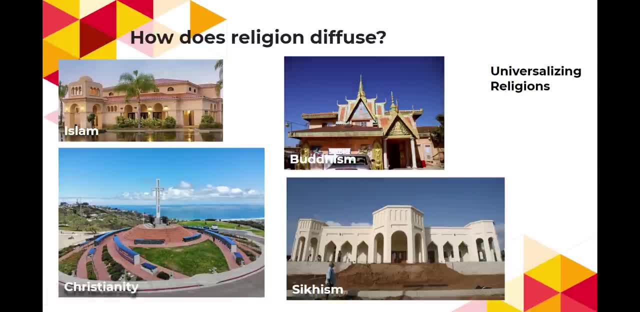 pronounce the word, but it's guru are something like that: sorry if I probably mispronounce that, I apologize but I'm trying. but these are different places of worship for these different universalizing religions and on, San Diego is a big enough city that we have adherence of all four of those religions. 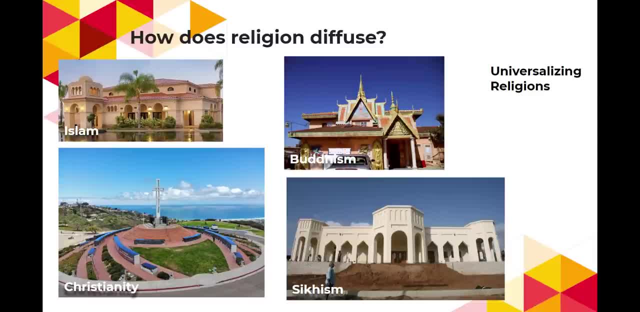 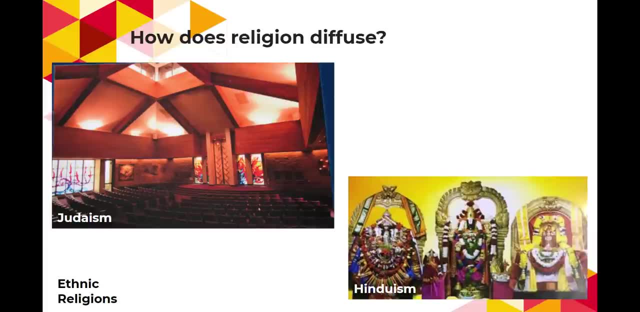 on here in this community and we can see examples of those religions across the landscape all right now. different from universalizing religions are ethnic religions. whereas universalizing religions are going to spread through not only relocation diffusion but expansion diffusion as well, ethnic religions typically only diffuse through relocation diffusion. 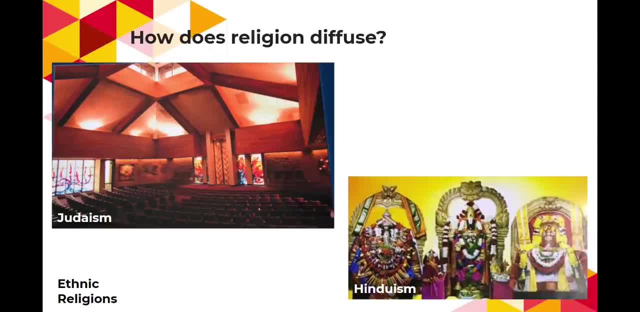 because ethical religions usually don't go out and try to convert other people to their religion. okay, and the two main examples we have that are Judaism and Hinduism, and these two places are also in San Diego but they're on the inside so you can't kind of, you know, wouldn't really count the inside as part of the. 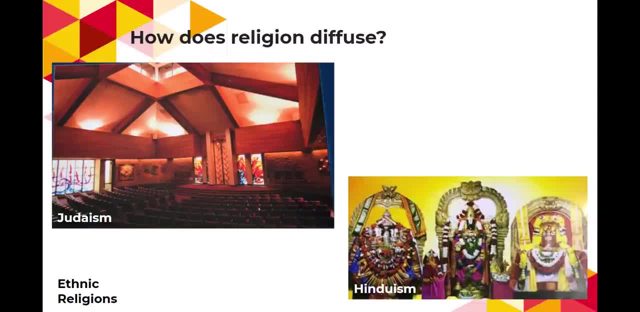 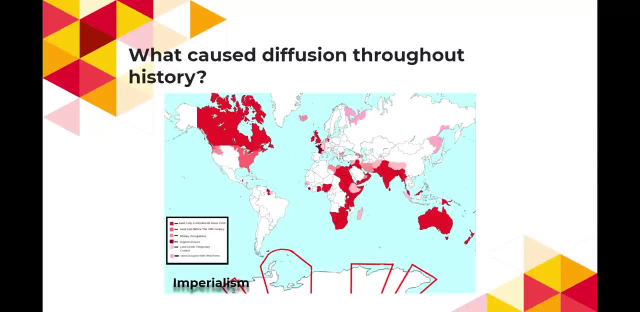 cultural landscape, but it is another example how Judaism and Hinduism have communities here in San Diego as well. all right, so let's talk about what has caused diffusion throughout history, and one of the big causers of diffusion has been imperialism. all right, this map shows us the extent of the influence of 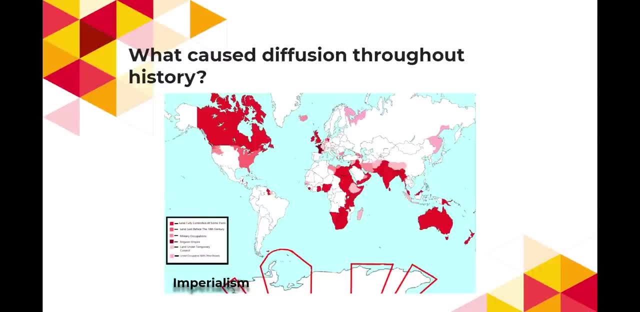 imperialism, all right. this map shows us the extent of the influence of imperialism. has been imperialism all right. this map shows us the extent of the influence of imperialism, all right. this map shows us the extent of the influence of imperialism. has been imperialism all right. this map shows us the extent of the influence of 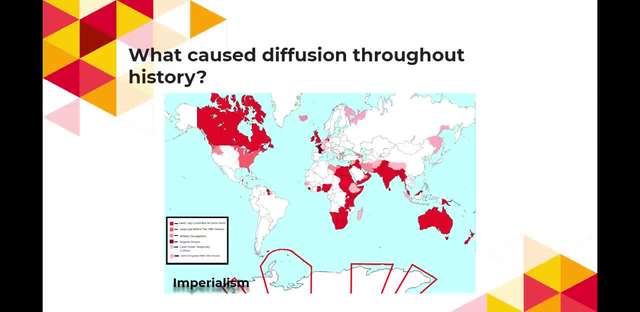 imperialism. all right, this map shows us the extent of the influence of imperialism of the British Empire. we see imperialism of the British Empire. we see imperialism of the British Empire. we see that word in a way and in the word, that word in a way and in the word. 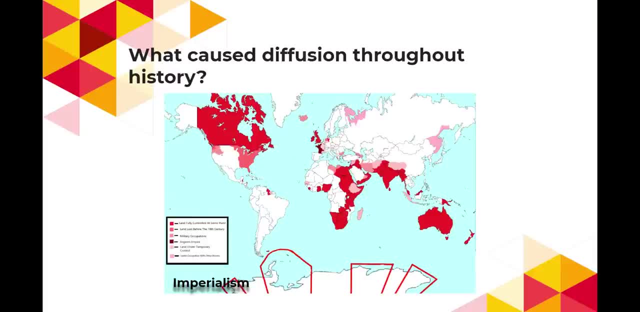 that word in a way, and in the word imperialism, we see Empire in there and imperialism, we see Empire in there and imperialism, we see Empire in there and imperialism is just a way. a country is imperialism is just a way a country is. imperialism is just a way a country is going to expand their reach beyond their. 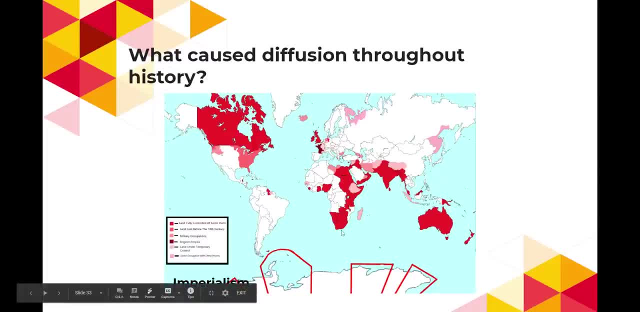 going to expand their reach beyond their, going to expand their reach beyond their borders. okay, so, um, you know, you know just borders. okay, so, um, you know, you know just borders. okay, so, um, you know, you know, just from being a member of the world, for, from being a member of the world for, 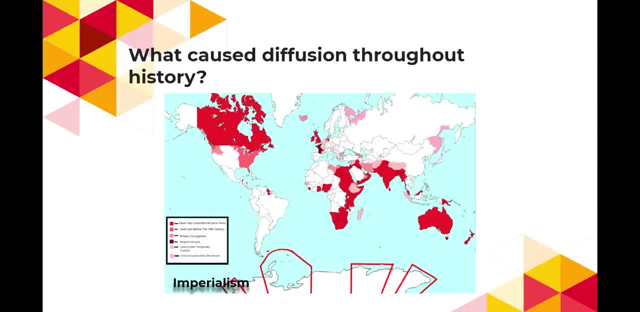 from being a member of the world for however long you've been alive, that, however long you've been alive, that, however long you've been alive, that English is spoken in a lot of different English is spoken in a lot of different. English is spoken in a lot of different places, not just in England, right um it. 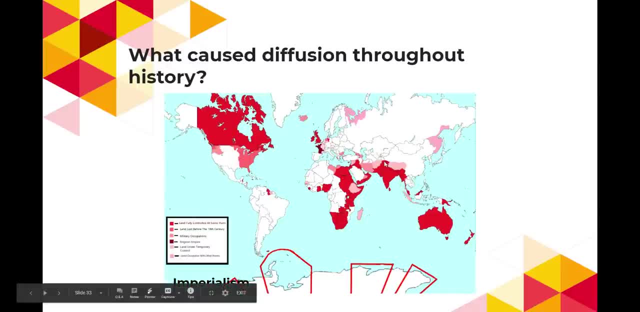 places, not just in England, right um, it places not just in England, right um, it is spoken here in the United States and is spoken here in the United States and is spoken here in the United States and Canada, in many parts of South Asia, in Canada, in many parts of South Asia, in. 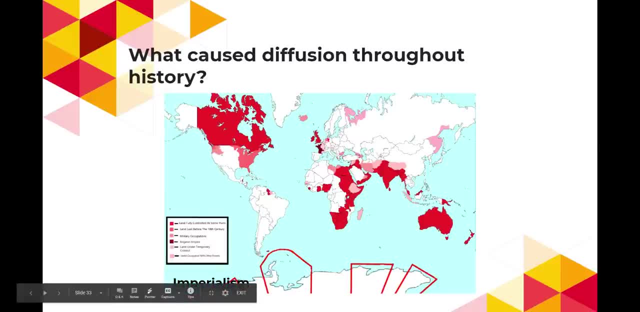 Canada, in many parts of South Asia, in Africa and Australia, and that goes back Africa and Australia, and that goes back Africa and Australia, and that goes back to the extent of the British Empire. so to the extent of the British Empire, so to the extent of the British Empire, so imperialism has been a big cause of. 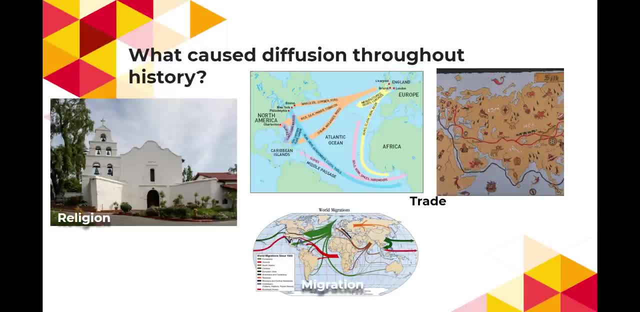 imperialism has been a big cause of imperialism has been a big cause of diffusion throughout history, um, but diffusion throughout history, um, but diffusion throughout history, um. but there's been other other causes as well. there's been other other causes as well. there's been other other causes as well, whether that is religion. here is the. 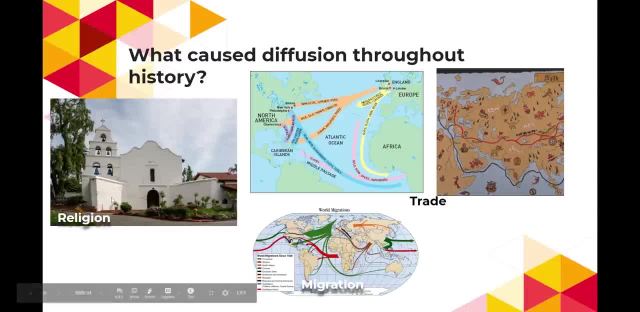 whether that is religion. here is the. whether that is religion. here is the Mission San Diego. this, you know, this is Mission San Diego. this, you know, this is Mission San Diego. this, you know, this is an example of how Christianity, an example of how Christianity, an example of how Christianity, Christianity diffused from Europe to the 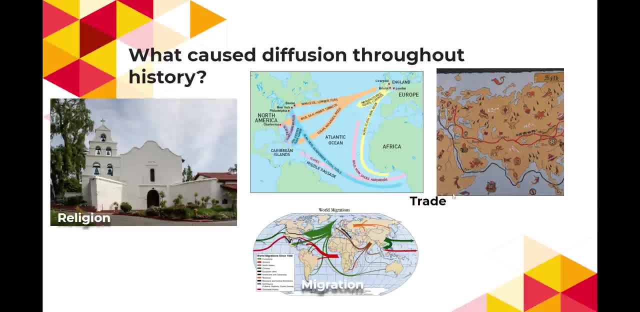 Christianity diffused from Europe to the Christianity diffused from Europe to the New World throughout history, or another New World throughout history, or another New World throughout history, or another example could be trade- whether we're example could be trade. whether we're example could be trade. whether we're trading, you know, innocuous items like 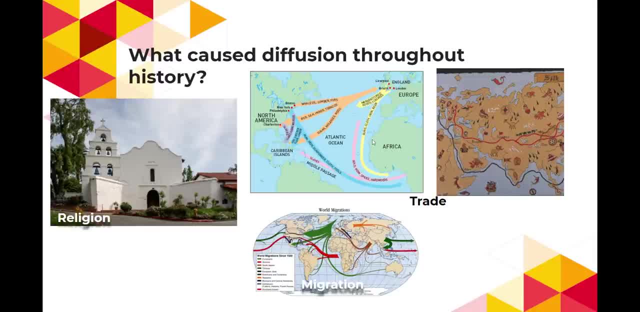 trading. you know innocuous items like trading. you know innocuous items like spices on the Silk Road. or we're doing spices on the Silk Road, or we're doing spices on the Silk Road, or we're doing what we, what we know now shouldn't be what we, what we know now, shouldn't be. 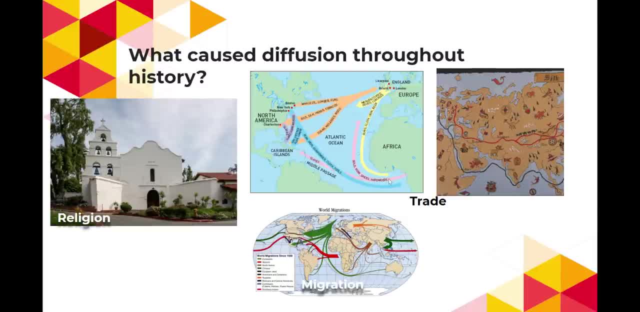 what we, what we know now, shouldn't be done at all and we're trading people done at all and we're trading people done at all and we're trading people through the slave trade and triangular, through the slave trade and triangular, through the slave trade and triangular trade across the Atlantic Ocean. 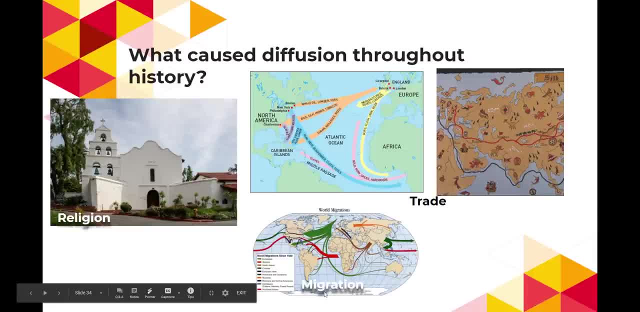 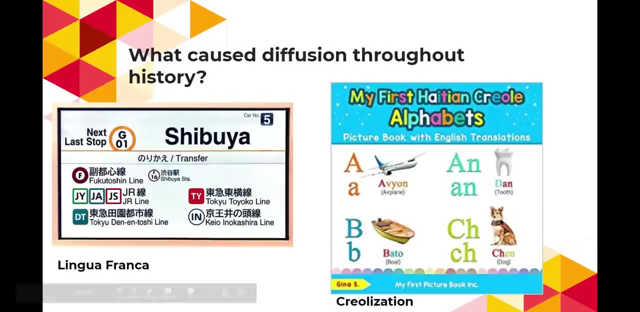 trade across the Atlantic Ocean. trade across the Atlantic Ocean. migration, as well has been a big cause. migration, as well, has been a big cause. migration as well has been a big cause of diffusion on just people moving from, of diffusion on just people moving from, of diffusion on just people moving from one place to the other. all right, as a 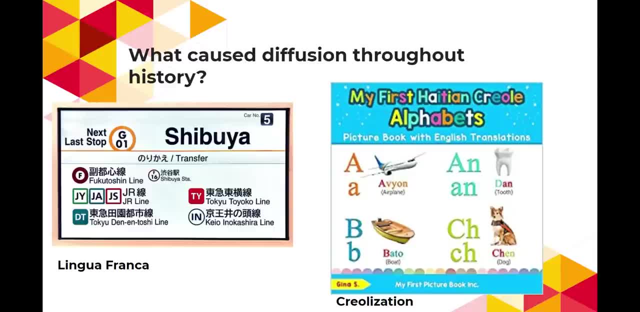 one place to the other, all right. as a one place to the other, all right. as a result of diffusion. we have a couple result of diffusion. we have a couple result of diffusion. we have a couple ideas that you need to know. one of those ideas that you need to know, one of those. 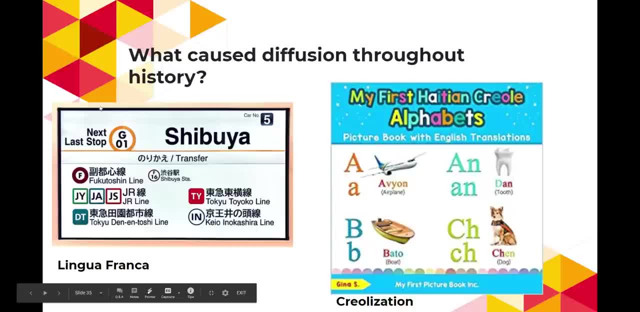 ideas that you need to know. one of those is lingua franca. so right here, you see, is lingua franca. so right here, you see, is lingua franca. so right here, you see this sign of a subway stop in Japan, okay, this sign of a subway stop in Japan, okay. 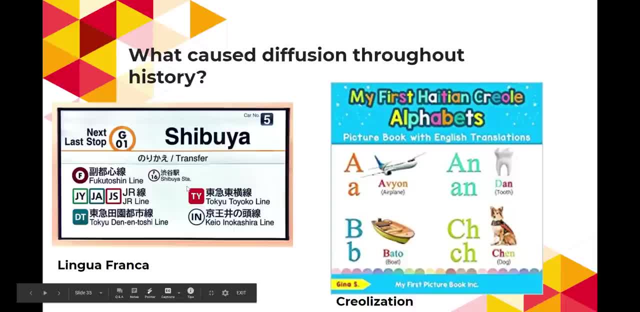 this sign of a subway stop in Japan. okay, Shibuya station, it would be near this Shibuya station. it would be near this Shibuya station, it would be near this place. and you see that this sign in place, and you see that this sign in place, and you see that this sign, in addition to being Japanese, is also in. 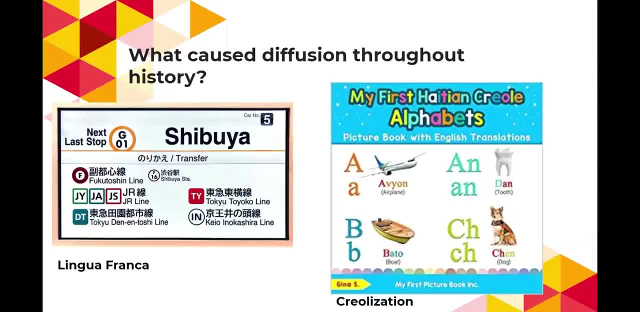 addition to being Japanese, is also, in addition to being Japanese, is also in English right, and that's because English English right, and that's because English English right, and that's because English is serves as a lingua franca and a lot is serves as a lingua franca and a lot. 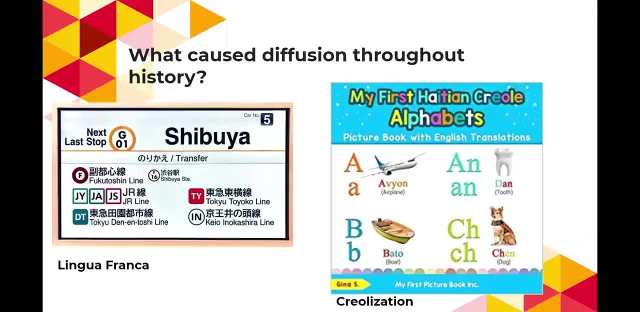 is serves as a lingua franca, and a lot of different parts around around our, of different parts around around our, of different parts around around our world. all right again going back to the world. all right again going back to the world. all right again. going back to the British Empire, going back to the extent. 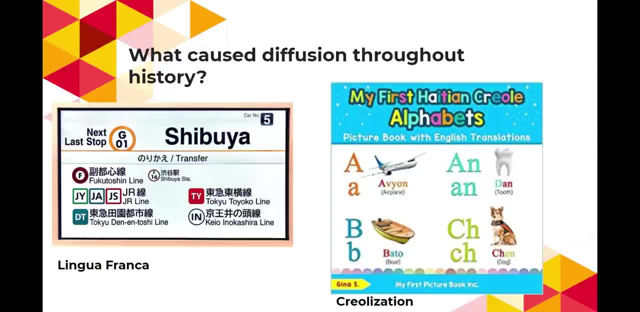 British Empire, going back to the extent British Empire, going back to the extent of that Empire and and also on the of that Empire, and and also on the of that Empire, and and also on the extent to not the American Empire, so to extent to not the American Empire, so to. 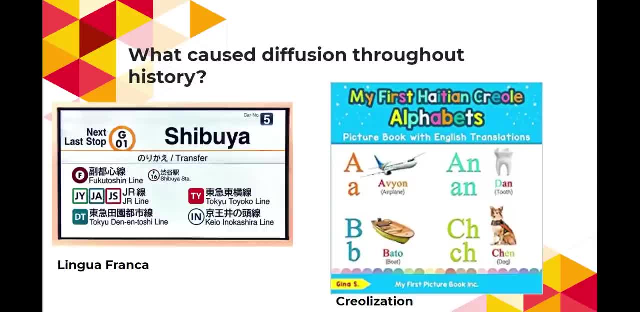 extent to not the American Empire, so to speak, but just how powerful you the speak, but just how powerful you the speak, but just how powerful you, the United States, has become in the last 200 United States has become in the last 200 United States has become in the last 200 years. okay, so in lots of different. 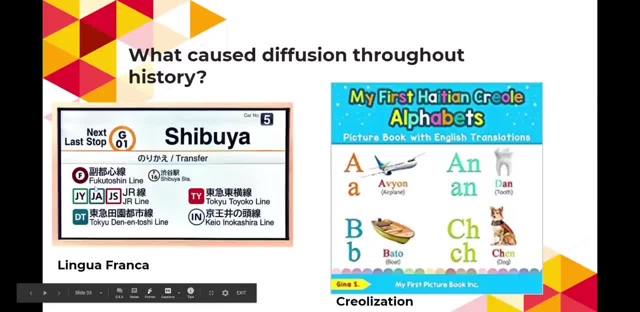 years. okay, so in lots of different years. okay, so in lots of different places, and not just Tokyo. but you see places and not just Tokyo. but you see places and not just Tokyo. but you see English used as a lingua franca, all. English used as a lingua franca, all. 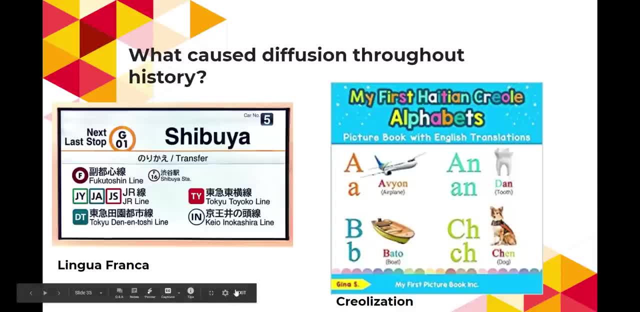 English used as a lingua franca, all right. another great example of what we right. another great example of what we right. another great example of what we get as a result of diffusion is get as a result of diffusion. is get as a result of diffusion. is creolization. okay, Haitian Creole is a creolization. okay, Haitian Creole is a creolization. okay, Haitian Creole is a language that's spoken primarily in language that's spoken primarily in language that's spoken primarily in Haiti, but in other parts of the world as Haiti, but in other parts of the world as. 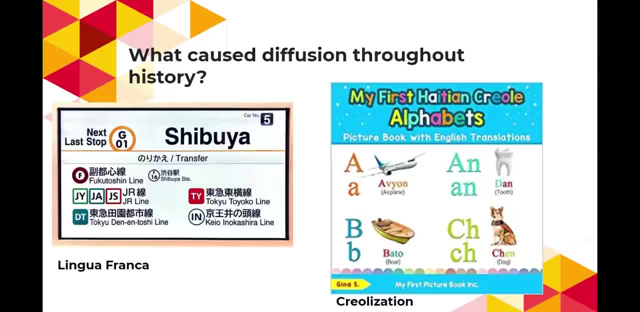 Haiti, but in other parts of the world as well, where you're taking different well, where you're taking different well, where you're taking different languages and combining them together to languages and combining them together to languages and combining them together to get something new, in this case, on 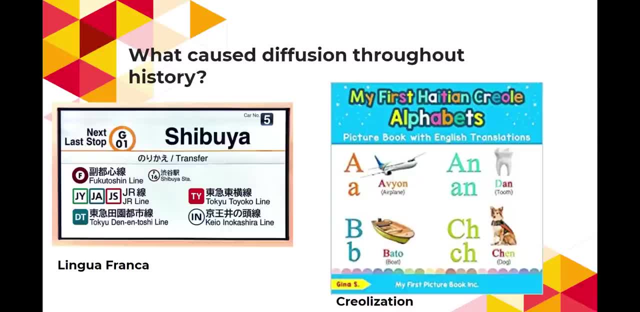 get something new in this case on. get something new in this case on: indigenous African languages are indigenous African languages are indigenous African languages. are combined with French to create Haitian. combined with French to create Haitian. combined with French to create Haitian Creole, which is kind of like a, like a. 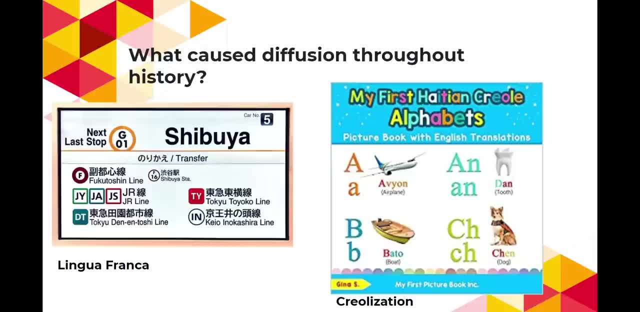 Creole, which is kind of like a like a Creole, which is kind of like a like a French, French inspired language. but it's French, French inspired language, but it's not really French. there's not really a not really French. there's not really a not really French. there's not really a lot of mutual intelligibility between. 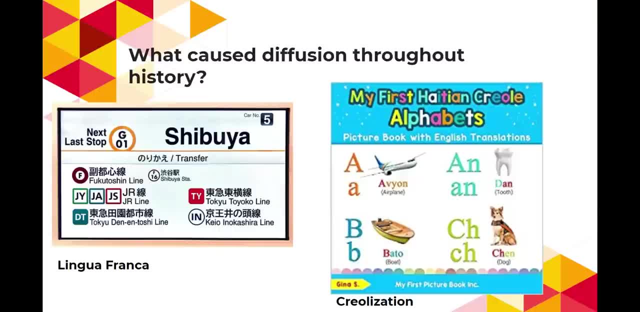 lot of mutual intelligibility between. lot of mutual intelligibility between Haitian Creole and French. meaning that a Haitian Creole and French. meaning that a Haitian Creole and French. meaning that a French speaker wouldn't necessarily French speaker, wouldn't necessarily French speaker wouldn't necessarily understand a Haitian Creole speaker, not. 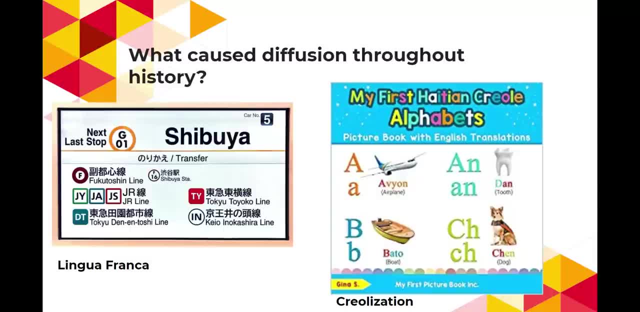 understand a Haitian Creole speaker. not understand a Haitian Creole speaker. not like how, when I speak Spanish, I can like how, when I speak Spanish, I can like how, when I speak Spanish, I can sort of sometimes understand someone who sort of sometimes understand someone who. 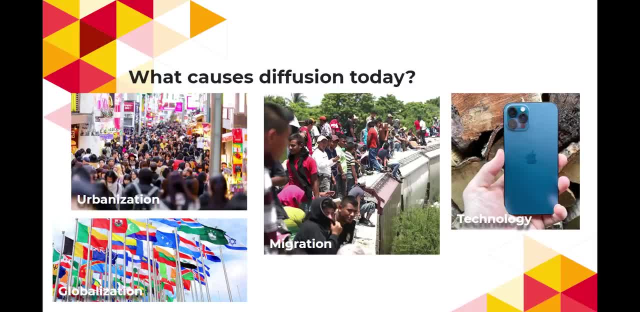 sort of sometimes understand someone who might be speaking Italian, although might be speaking Italian, although might be speaking Italian, although usually to work all right. what usually to work all right? what usually to work all right. what causes of diffusion today? let's talk. causes of diffusion today, let's talk. 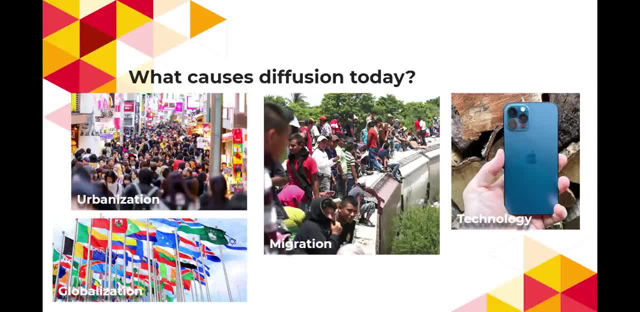 causes of diffusion. today, let's talk about contemporary positive diffusion. we about contemporary positive diffusion. we about contemporary positive diffusion. we see things like urbanization, or see things like urbanization, or see things like urbanization, or essentially the growth of cities and the, essentially the growth of cities and the. 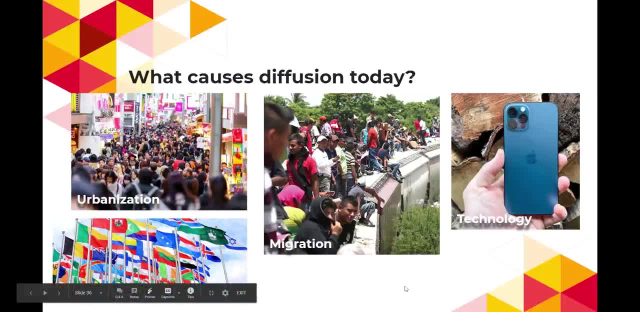 essentially the growth of cities and the movement of people towards cities. we movement of people towards cities. we movement of people towards cities. we also see globalization, or the idea that also see globalization, or the idea that also see globalization, or the idea that already our ideas can get around the. 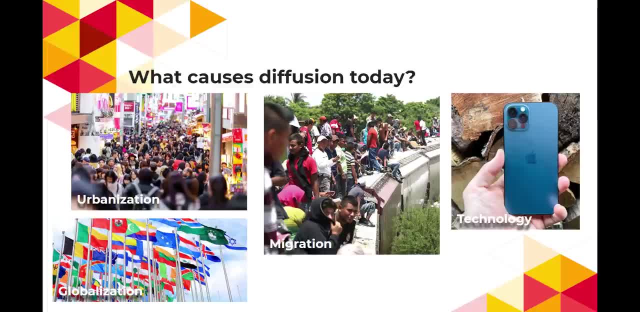 already our ideas can get around the already our ideas can get around the globe in a very fast manner. now because globe in a very fast manner now, because globe in a very fast manner now because of things like technology, like the of things like technology, like the of things like technology like the iphone. okay, migration, uh, you'll see, is 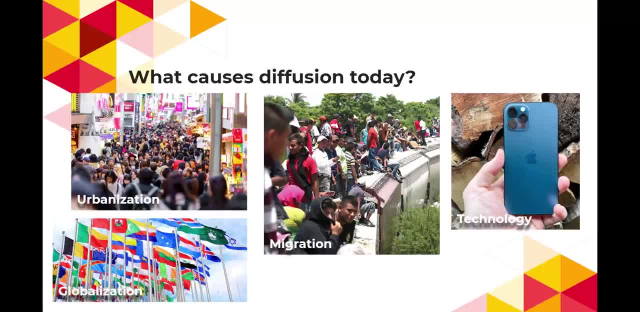 iphone, okay, migration, uh, you'll see. is iphone, okay, migration, uh, you'll see, is also still on this slide. because it's also still on this slide, because it's also still on this slide, because it's not just a historical cause of diffusion, not just a historical cause of diffusion. 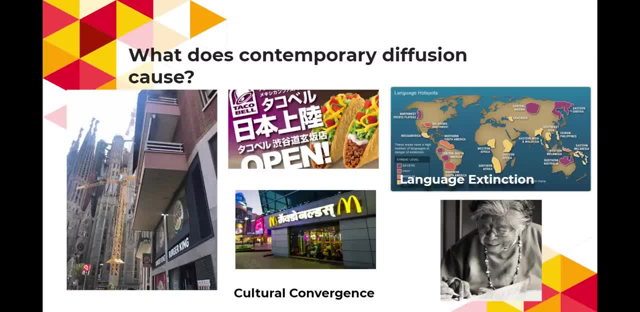 not just a historical cause of diffusion, but it's a contemporary cause of, but it's a contemporary cause of, but it's a contemporary cause of diffusion as well. diffusion as well. diffusion as well. all right now, what does contemporary all right now, what does contemporary all right now, what does contemporary diffusion cause? we see cultural. 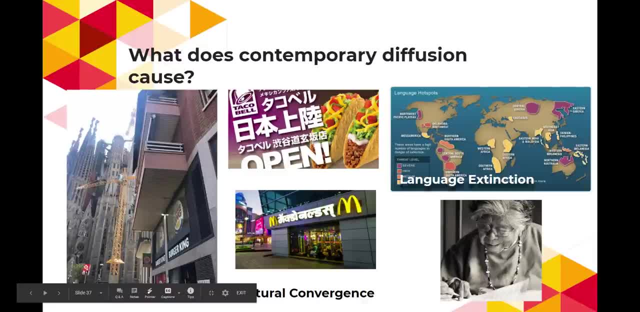 diffusion cause. we see cultural diffusion cause. we see cultural convergence. all right, this is the idea: convergence, all right. this is the idea. convergence, all right. this is the idea that our cultures are becoming more and that our cultures are becoming more and that our cultures are becoming more and more alike, more and more the same. okay. 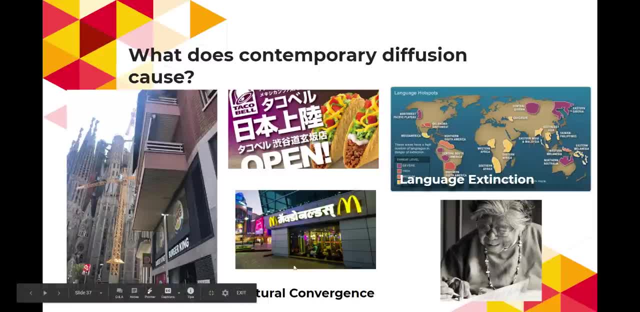 more alike, more and more the same, okay. more alike, more and more the same, okay. and you see that um with these examples, and you see that um with these examples, and you see that um with these examples of american fast food places in places, of american fast food places in places. 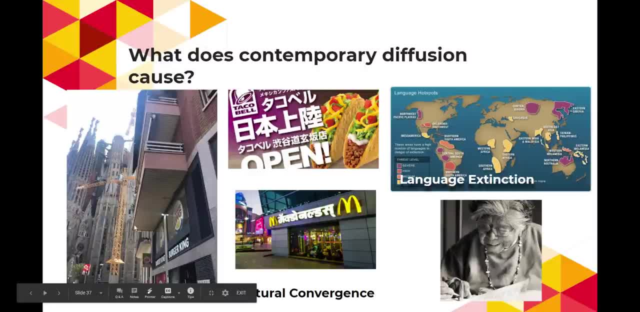 of american fast food places in places that are not america, whether it's this that are not america, whether it's this that are not america, whether it's this burger king across the street from la burger king, across the street from la burger king, across the street from la sagrada familia in barcelona, um or these. 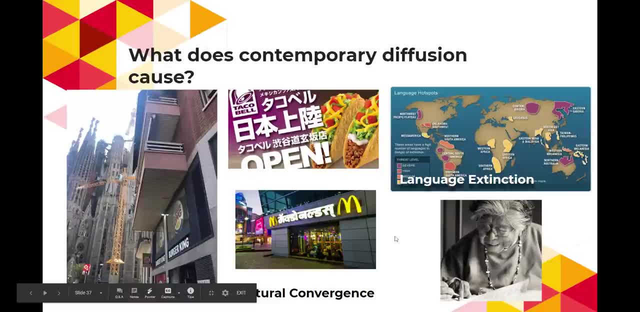 sagrada familia in barcelona, um, or these sagrada familia in barcelona, um, or these taco bells and mcdonald's in different taco bells and mcdonald's in different taco bells and mcdonald's in different parts of asia. okay, another example of 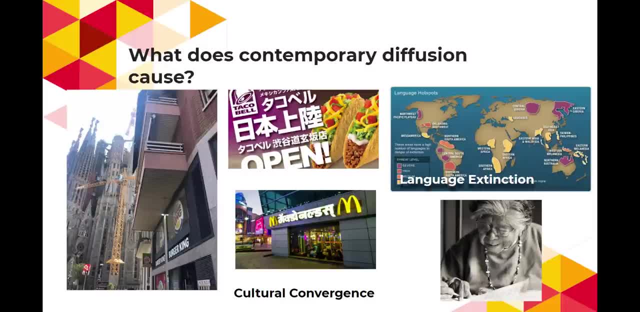 parts of asia. okay, another example of parts of asia. okay, another example of language. or just as a lingua franca: they language. or just as a lingua franca, they language, or just as a lingua franca. they have less of a reason, a reason to talk, have less of a reason, a reason to talk. 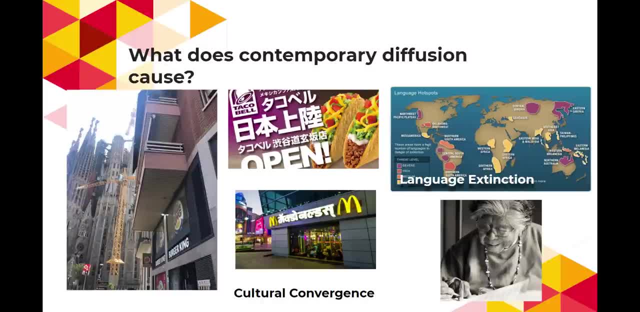 have less of a reason, a reason to talk about their own native language or their, about their own native language or their about their own native language or their own indigenous language. so you're seeing own indigenous language, so you're seeing own indigenous language. so you're seeing some languages die out, in fact the 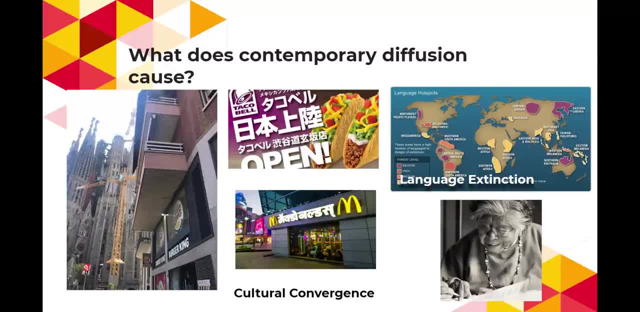 some languages die out. in fact, the some languages die out. in fact. the experts predict, experts predict. experts predict um that about every two weeks. we use um that about every two weeks. we use um that about every two weeks. we use one language off of the face of the earth. 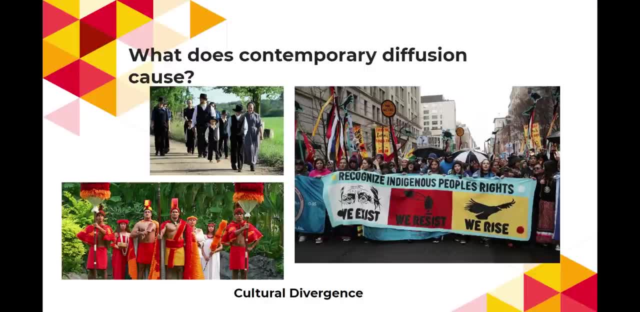 one language off of the face of the earth. one language off of the face of the earth, all right um. you also see cultural, all right um. you also see cultural, all right um. you also see cultural divergence as well. divergence as well, divergence as well um. some people, especially those people um. 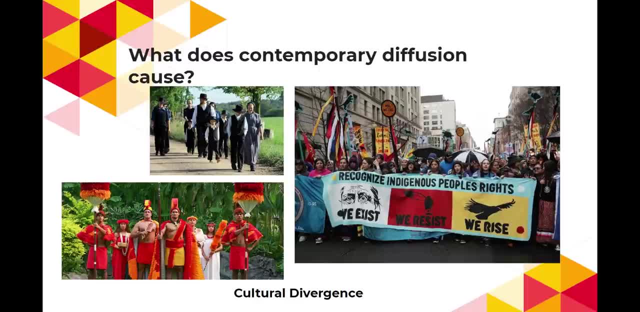 um some people, especially those people um um some people, especially those people um who are indigenous, who are indigenous, who are indigenous, whether they're native americans or whether they're native americans, or whether they're native americans or indigenous to another part of the world. 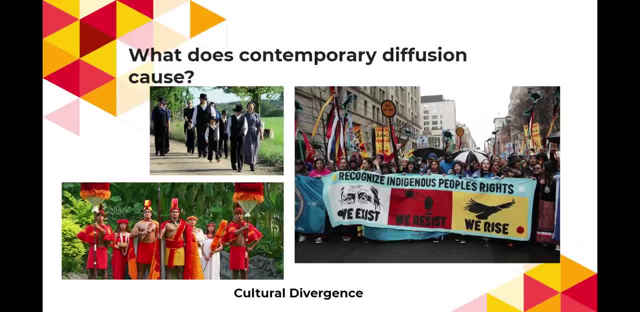 indigenous to another part of the world. indigenous to another part of the world. they're, they're kind of afraid of this. they're, they're kind of afraid of this. they're, they're kind of afraid of this. cultural convergence because they see it. cultural convergence because they see it. 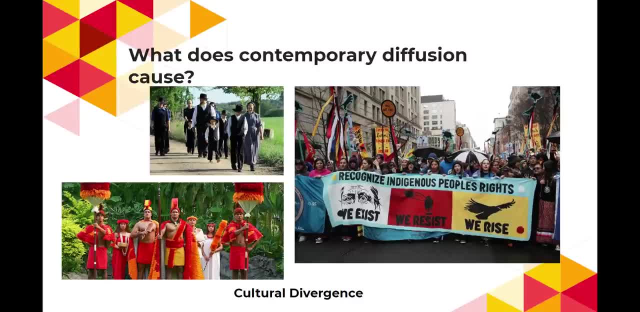 cultural convergence because they see it as a threat, as a threat, as a threat. they see that this americanization is. they see that this americanization is. they see that this americanization is going to cause their own native um, going to cause their own native um, going to cause their own native um culture to kind of die out. so they might. 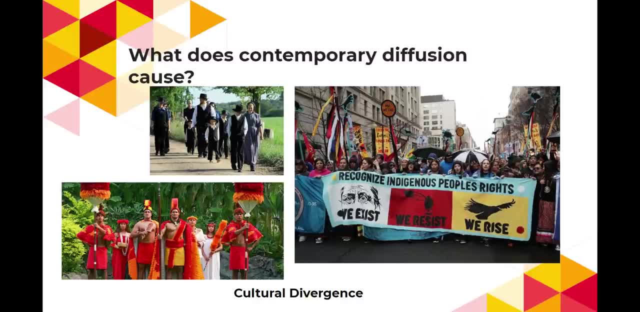 culture to kind of die out, so they might. culture to kind of die out, so they might take extra steps to preserve their own. take extra steps to preserve their own. take extra steps to preserve their own indigenous culture, indigenous culture, indigenous culture, um which could cause cultural, um which could cause cultural. 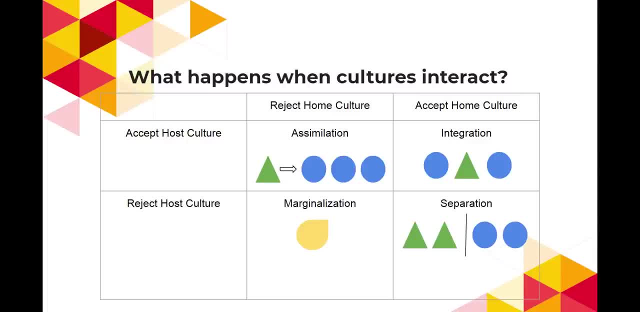 um, which could cause cultural divergence. divergence, divergence, all right. so what happens when cultures all right? so what happens when cultures all right? so what happens when cultures interact? so this is called interact. so this is called interact. so this is called barry's acculturation model. this was. 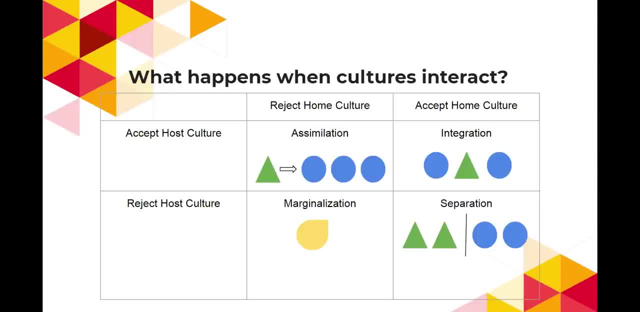 barry's acculturation model. this was barry's acculturation model. this was developed by developed by developed by um a social scientist named john barry. um a social scientist named john barry. um a social scientist named john barry and he studied what would happen to. 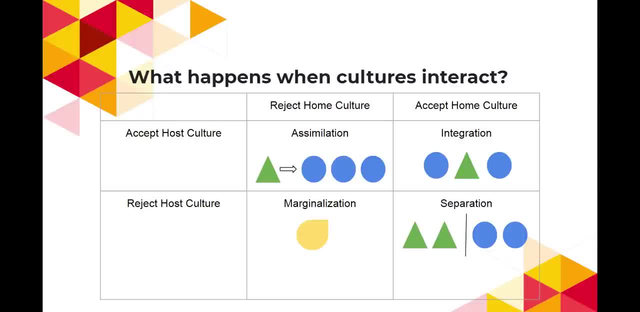 and he studied what would happen to. and he studied what would happen to people when they moved from one place to people, when they moved from one place to people, when they moved from one place to another, another, another, and there was two dichotomies that he 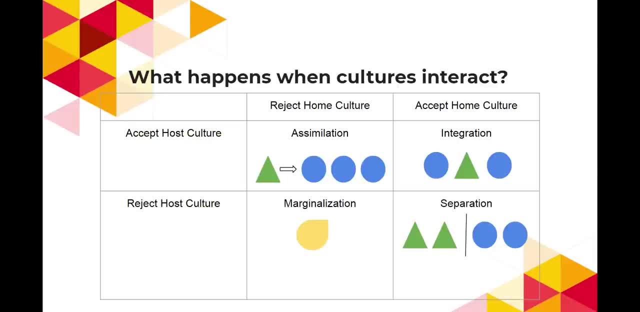 and there was two dichotomies that he and there was two dichotomies that he focused on- focused on. focused on um one of those being whether the person um one of those being whether the person um one of those being whether the person would. 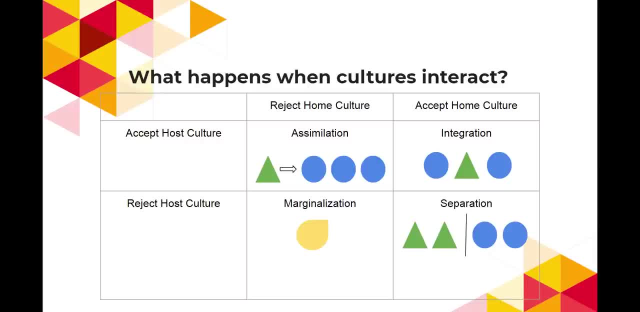 would would reject or accept the new culture. the reject or accept the new culture. the reject or accept the new culture. the culture, the place that they're going to, culture, the place that they're going to, culture, the place that they're going to, and whether they would reject or accept. 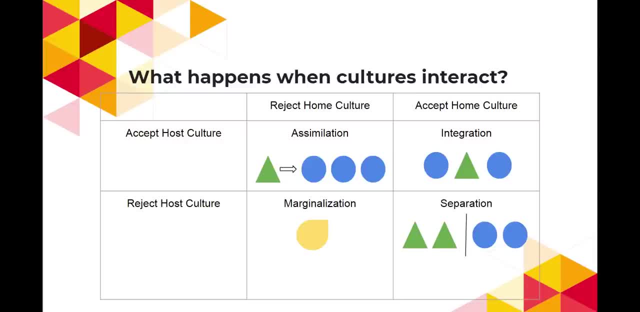 and whether they would reject or accept, and whether they would reject or accept um their host culture or their origin, um their host culture or their origin, um their host culture or their origin. culture right, the culture where they're culture right the culture where they're culture right, the culture where they're, that they're coming from. 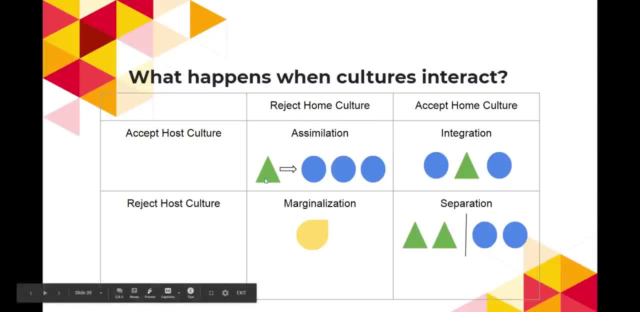 that they're coming from. that they're coming from if you're rejecting the home culture and if you're rejecting the home culture and if you're rejecting the home culture and accepting the host culture. that's what accepting the host culture, that's what accepting the host culture, that's what we call assimilation. 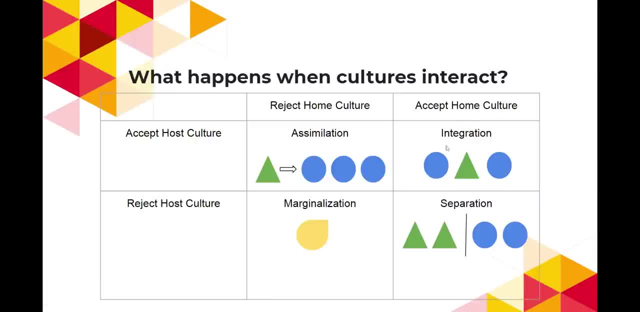 we call assimilation. we call assimilation: all right if you're accepting both of. all right if you're accepting both of all right if you're accepting both of them. that sounds pretty good to me. them, that sounds pretty good to me. them, that sounds pretty good to me. we would call that integration, um, if 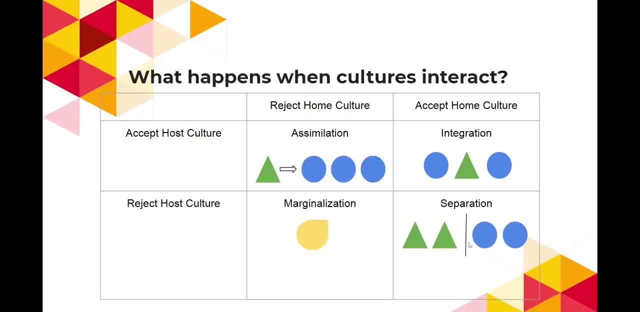 we would call that integration um. if we would call that integration um. if you're accepting the home culture but you're accepting the home culture, but you're accepting the home culture but rejecting your host culture, rejecting your host culture, rejecting your host culture, we would call that separation. and if 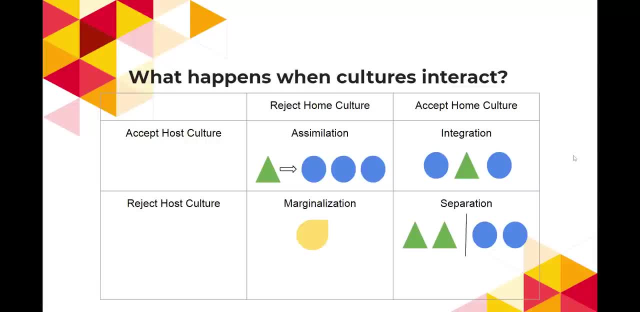 we would call that separation. and if we would call that separation, and if you're rejecting both of those, you're rejecting both of those, you're rejecting both of those. that would be marginalization, all right, that would be marginalization, all right, that would be marginalization, all right. so for assimilation, i have this um: 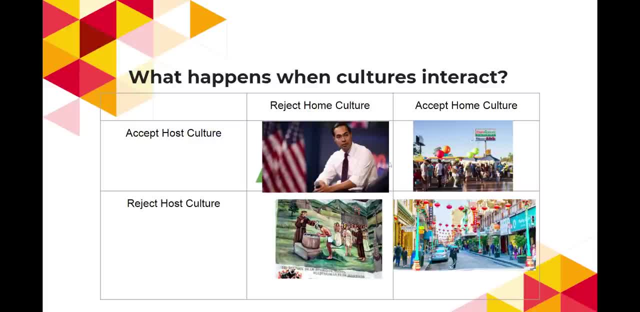 so, for assimilation, i have this: um. so, for assimilation, i have this: um image of julian castro, who was a image of julian castro, who was a image of julian castro, who was a presidential candidate, presidential candidate, presidential candidate um, and the former mayor of san antonio. 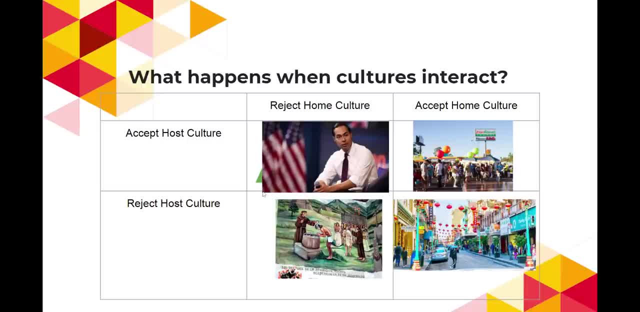 um and the former mayor of san antonio um and the former mayor of san antonio don't speak the best spanish um and we don't speak the best spanish um and we don't speak the best spanish um. and we called that assimilation, called that assimilation. 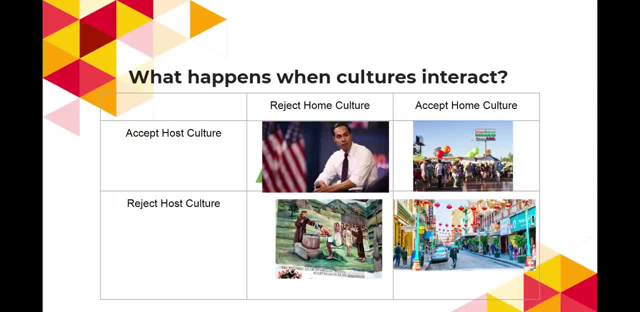 called that assimilation um, and we see that with a lot of mexican um, and we see that with a lot of mexican um, and we see that with a lot of mexican americans, americans, americans, um, and they're slowly starting to speak. 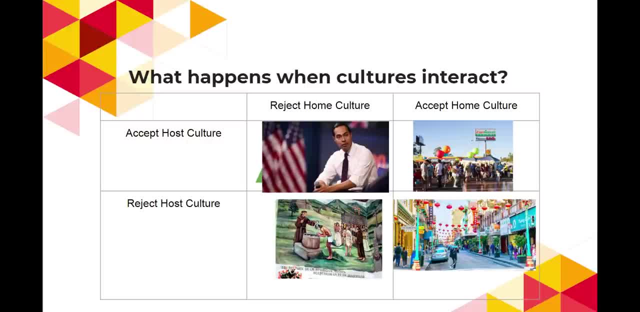 um, and they're slowly starting to speak. um, and they're slowly starting to speak a little bit less and less spanish, a little bit less and less spanish, a little bit less and less spanish, as more and more generations are born, as more and more generations are born. 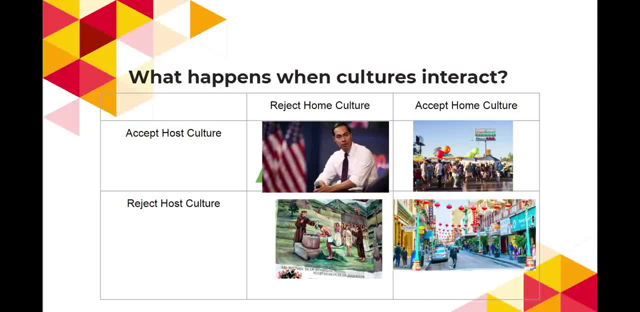 as more and more generations are born here in the united states, there some here in the united states, there some here in the united states, there some some mexican-american families might some mexican-american families, might some mexican-american families might, lose those ties back to their 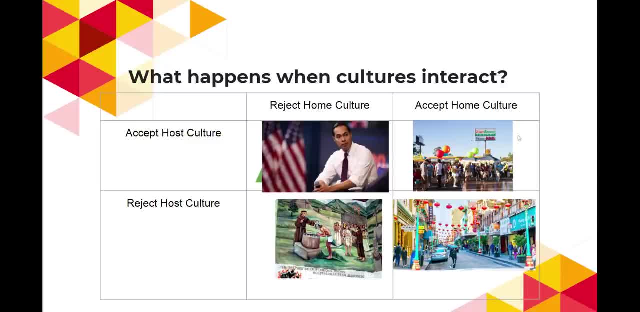 lose those ties back to their, lose those ties back to their traditional mexican culture, traditional mexican culture, traditional mexican culture. all right now if you're accepting both. all right now if you're accepting both. all right now if you're accepting both the home culture and your host culture. 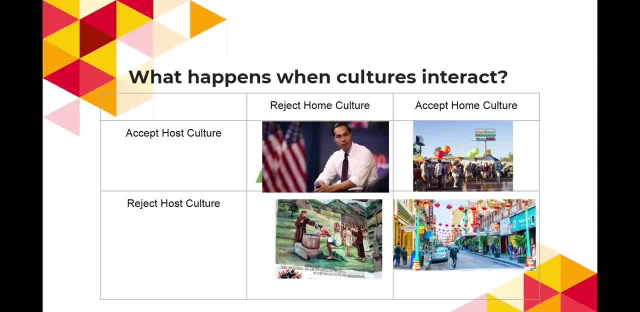 the home culture and your host culture. the home culture and your host culture- um uh, we would call that integration and um uh, we would call that integration and um uh, we would call that integration, and that might be, that might be, that might be some sort of celebration of the culture. some sort of celebration of the culture, some sort of celebration of the culture of the place where you're coming from, of the place where you're coming from, of the place where you're coming from, but also still being able to integrate, but also still being able to integrate. 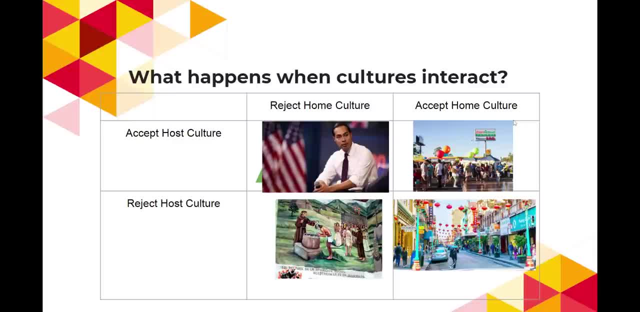 but also still being able to integrate within the new culture, within the new culture, within the new culture, and the example i have here is um it was. and the example i have here is um it was. and the example i have here is um it was an image of the san diego night market. 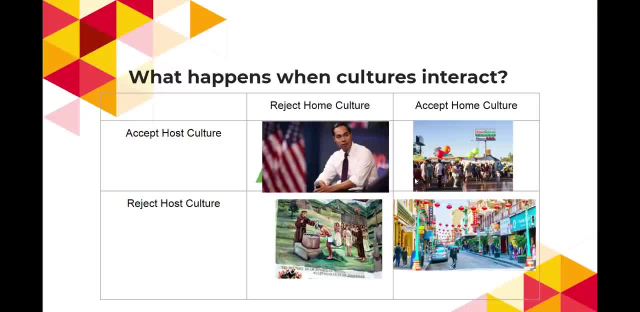 an image of the san diego night market. an image of the san diego night market. this, this, this picture is not at night. obviously um picture is not at night. obviously um picture is not at night, obviously, um. but it's a festival that you know, but it's a festival that you know. 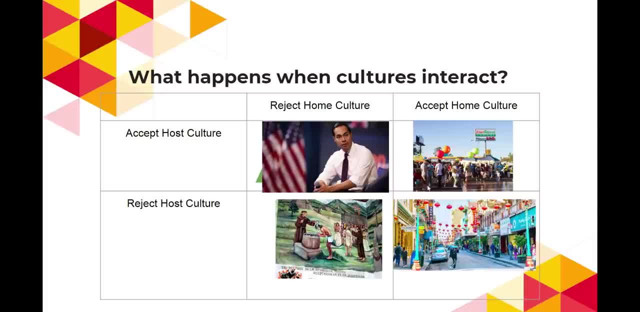 but it's a festival that you know before covid used to happen in the. before covid used to happen in the. before covid used to happen in the convoy era. convoy era- convoy era. area of san diego where people could come. area of san diego where people could come. 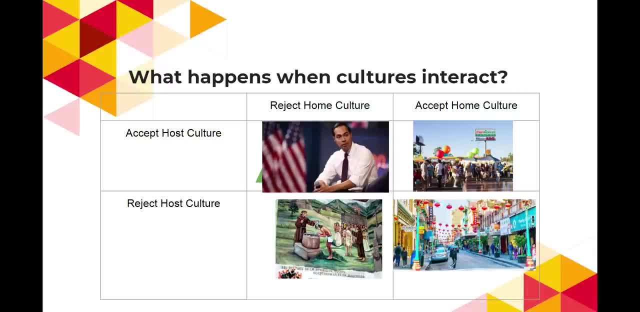 area of san diego where people could come and enjoy and enjoy and enjoy um more traditional asian food, but then um more traditional asian food, but then um more traditional asian food. but then you know that place is right in the. you know that place is right in the. 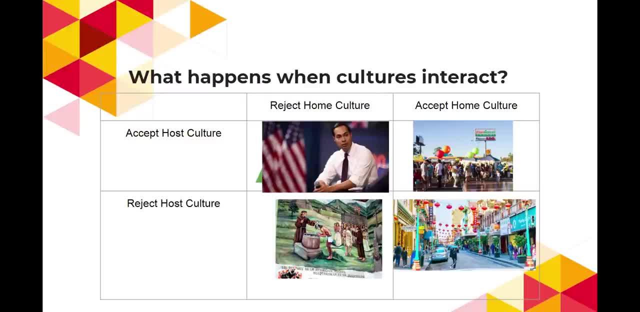 you know that place is right in the middle of the united states and middle of the united states and middle of the united states. and um you know you're still accepting that, um you know you're still accepting that, um you know you're still accepting that home culture. 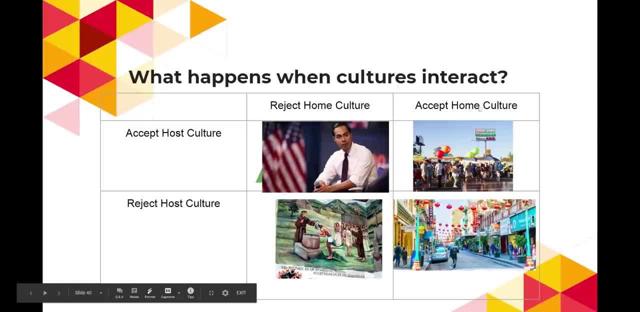 home culture, home culture. okay if you are accepting the home. okay if you are accepting the home. okay if you are accepting the home culture, culture, culture. you're the whole the culture from the. you're the whole the culture from the. you're the whole the culture from the place you came from. but rejecting the. 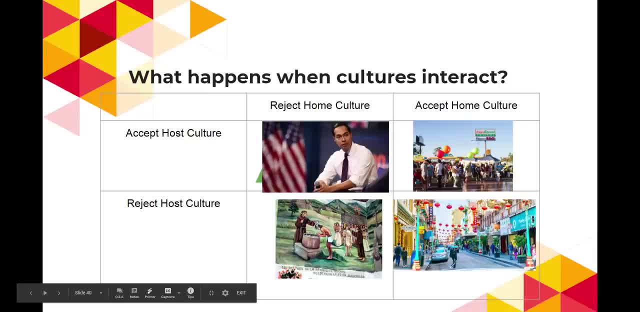 place you came from, but rejecting the place you came from, but rejecting the new culture, new culture, new culture. we would call that separation all right. we would call that separation all right. we would call that separation all right. and i have this image of chinatown and i have this image of chinatown. 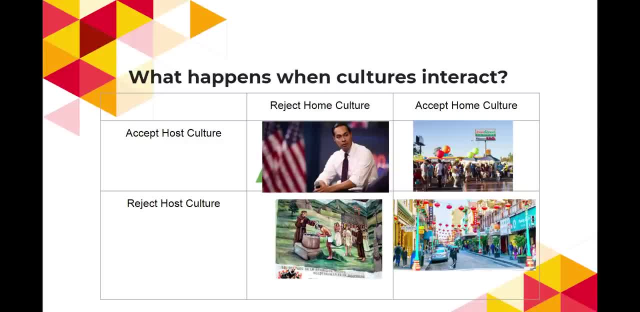 and i have this image of chinatown in san francisco because if you are an in san francisco, because if you are an in san francisco, because if you are an immigrant from china and you move to immigrant from china and you move to immigrant from china and you move to chinatown in the san francisco bay area, chinatown in the san francisco bay area, chinatown in the san francisco bay area, but then you kind of limit yourself to, but then you kind of limit yourself to, but then you kind of limit yourself to that neighborhood and you never learn that neighborhood and you never learn. 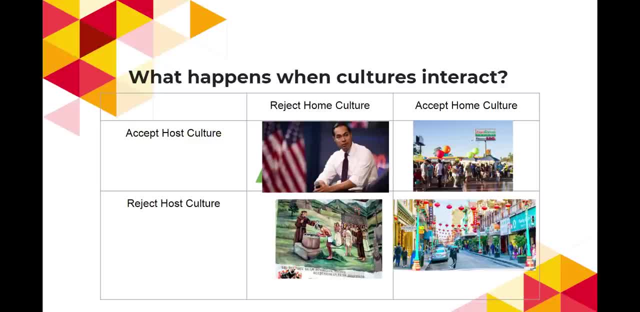 that neighborhood and you never learn english, or you never eat more english, or you never eat more english, or you never eat more traditional american foods, or you never traditional american foods, or you never traditional american foods, or you never do anything to to integrate yourself. do anything to to integrate yourself. 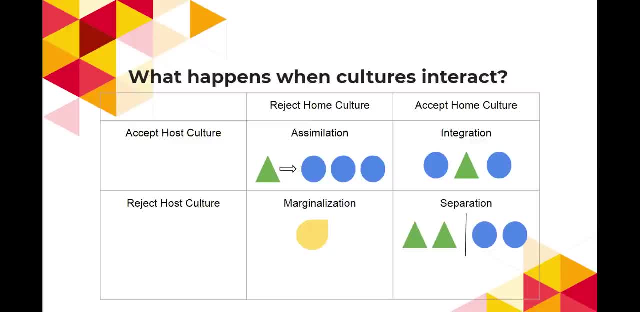 do anything to, to integrate yourself with american culture, that would be with american culture, that would be with american culture. that would be called um, called um, called um. separation okay, separation, okay, separation, okay. and the last one here is when you're, and the last one here is when you're. 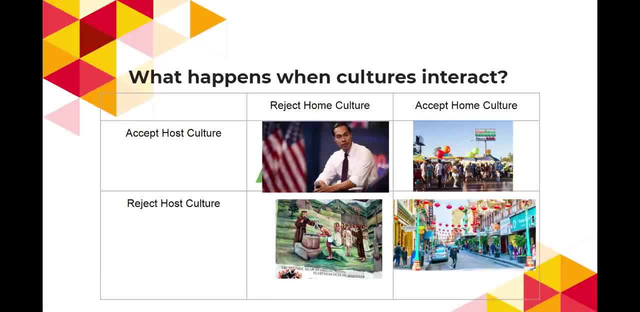 and the last one here is when you're rejecting both of them, and a good rejecting both of them and a good rejecting both of them, and a good example of that is the forced conversion. example of that is the forced conversion. example of that is the forced conversion of the aztecs. so this is like a 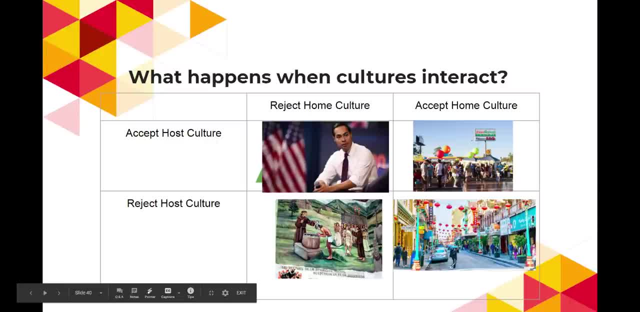 of the aztecs. so this is like a of the aztecs. so this is like a, an image of of that. not you know an image of of that. not you know an image of of that, not you know. obviously it's a painting, um, obviously it's a painting um. 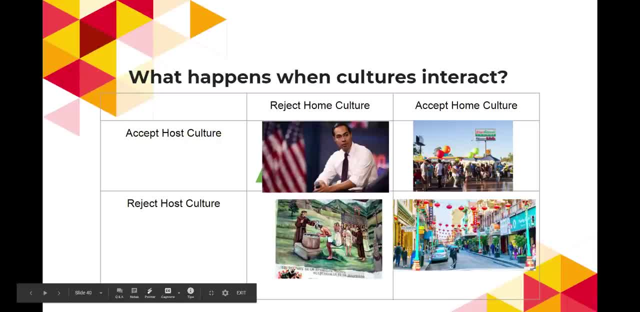 obviously it's a painting, um, but, but. but. after hernan cortez and the conquistadors, after hernan cortez and the conquistadors, after hernan cortez and the conquistadors came and defeated the aztec empire, came and defeated the aztec empire. 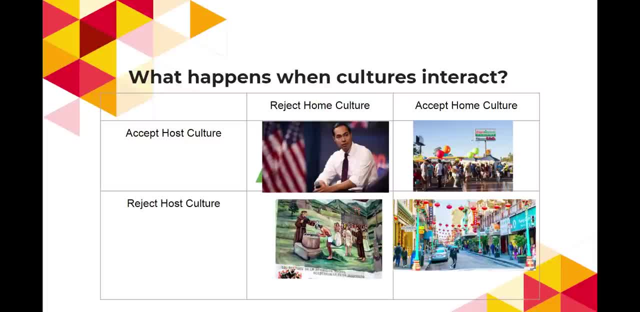 came and defeated the aztec empire. they forced those people to convert to. they forced those people to convert to. they forced those people to convert to catholicism, to convert to christianity, catholicism to convert to christianity, catholicism to convert to christianity. so they can no longer celebrate their 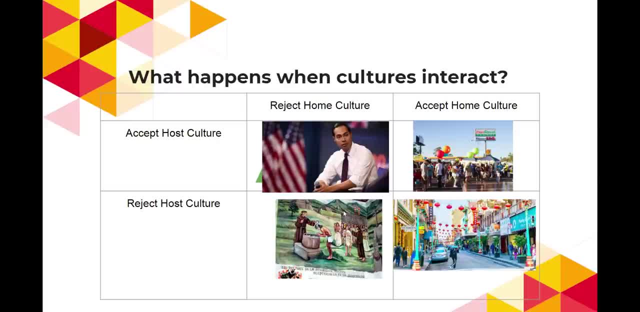 so they can no longer celebrate their, so they can no longer celebrate their traditional aztec culture, traditional aztec culture, traditional aztec culture. and since they were forced to convert, and since they were forced to convert, and since they were forced to convert, they probably didn't weren't too happy. 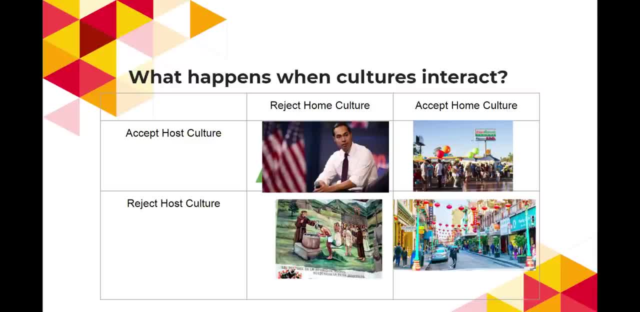 they probably didn't weren't too happy. they probably didn't weren't too happy with their new culture either with their new culture, either with their new culture either. and we call that marginalization, not a, and we call that marginalization, not a. and we call that marginalization not a very good situation. 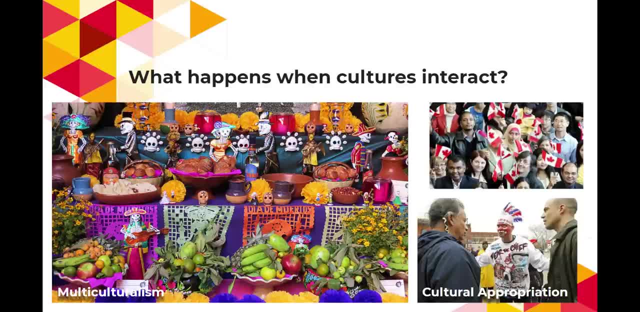 very good situation. very good situation, all right. what happens when cultures? all right. what happens when cultures? all right. what happens when cultures interact, interact, interact- uh, we can get things like multiculturalism. uh, we can get things like multiculturalism. uh, we can get things like multiculturalism. all right, you're seeing more and more. 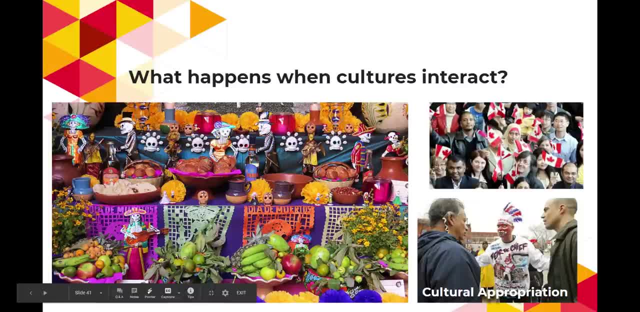 all right, you're seeing more and more. all right, you're seeing more and more places around the united states. places around the united states. places around the united states. celebrate dia de los muertos, uh right. celebrate dia de los muertos, uh right. celebrate dia de los muertos, uh right, after halloween. 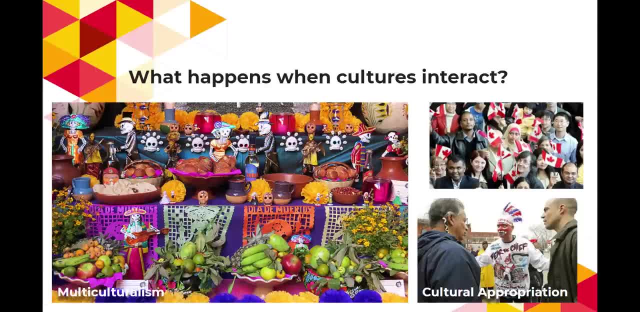 after halloween: after halloween, uh, it's the celebration of of our uh. it's the celebration of of our uh, it's the celebration of of our ancestors that comes from traditional ancestors, that comes from traditional ancestors, that comes from traditional mexican culture, but it's also a. 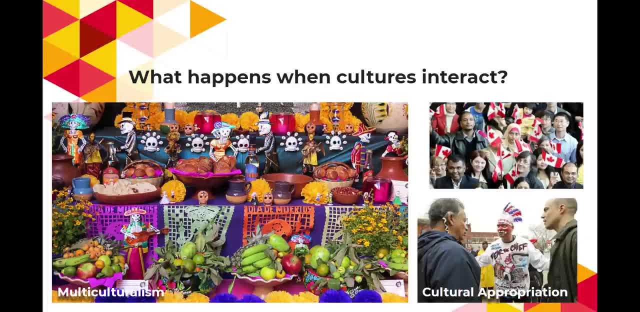 mexican culture, but it's also a mexican culture, but it's also a combination, combination, combination of of not only indigenous culture, but of, of not only indigenous culture, but of of not only indigenous culture, but some elements of catholicism as well, some elements of catholicism as well. 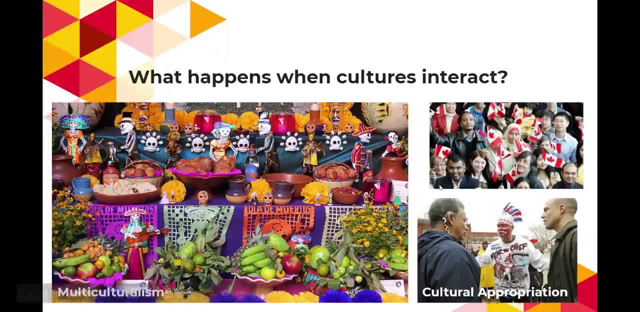 some elements of catholicism as well. okay, canada is a great example of a. okay, canada is a great example of a. okay, canada is a great example of a multicultural place, multicultural place, multicultural place. lots of immigrants from other places, lots of immigrants from other places, lots of immigrants from other places that um integrate very seamlessly. 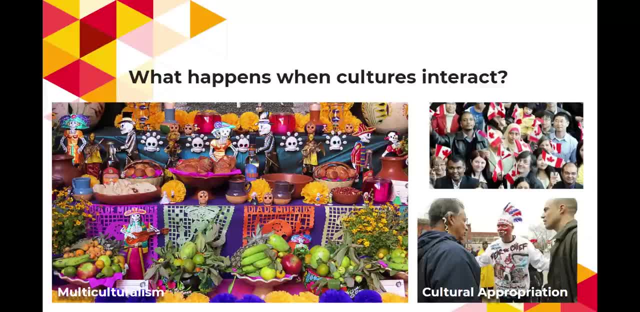 that um integrate very seamlessly, that um integrate very seamlessly in the canadian culture. but then you in the canadian culture, but then you in the canadian culture, but then you could go too far, could go too far, could go too far. where you might be like trying on, where you might be like trying on. 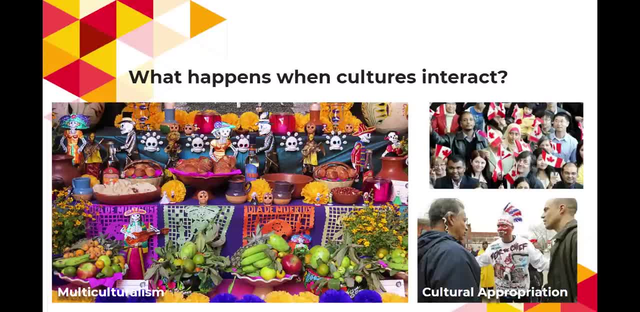 where you might be like trying on different cultures, different cultures, different cultures in a disrespectful way, and that's what in a disrespectful way, and that's what in a disrespectful way, and that's what we call cultural appropriation. we call cultural appropriation, we call cultural appropriation. um, like we see right here with this white. 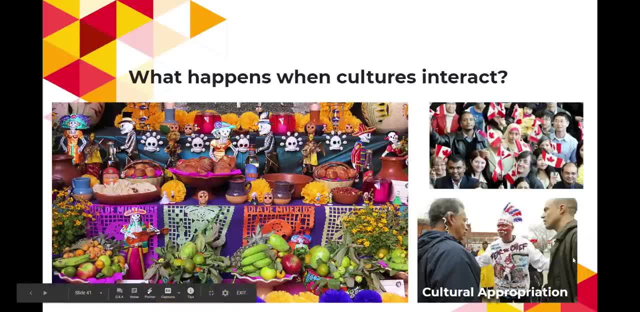 um, like we see right here with this white, um, like we see right here with this white person, person, person, um kind of degrading native american, um kind of degrading native american, um kind of degrading native american culture, culture, culture. uh, in the name of just supporting the 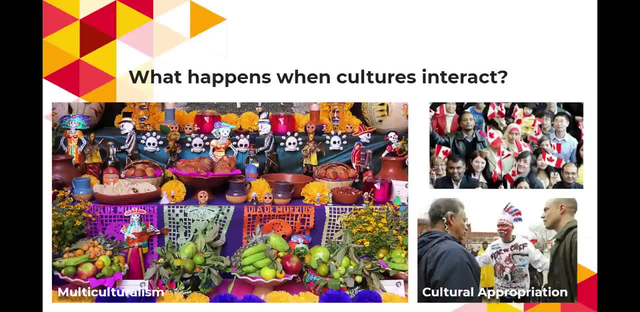 uh, in the name of just supporting the uh, in the name of just supporting the cleveland indians the sports team. so cleveland indians the sports team. so cleveland indians, the sports team. so, um can i advise this to not do that? um, can i advise this to not do that? 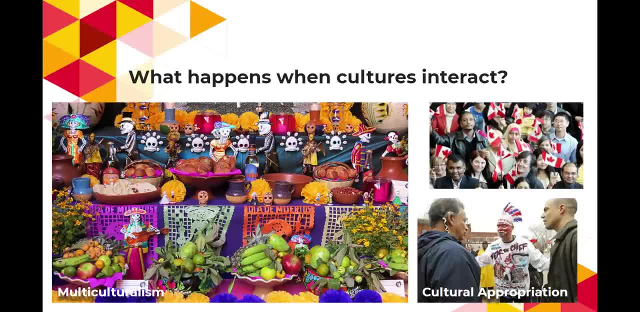 um, can i advise this to not do that. all right, that is it for unit three. all right, that is it for unit three. all right, that is it for unit three. ladies and gentlemen, ladies and gentlemen, ladies and gentlemen, thanks so much for being here. thanks so, thanks so much for being here, thanks so. 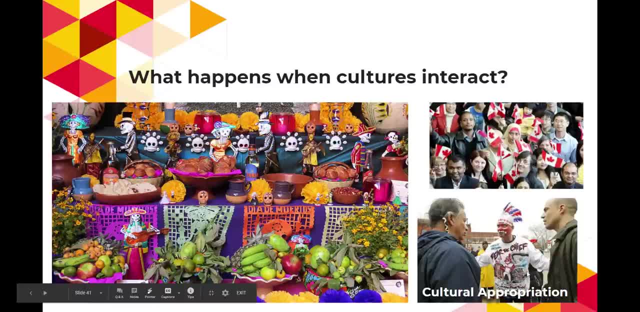 thanks so much for being here. thanks so much for watching the video. much for watching the video. much for watching the video. uh, don't forget to like and subscribe. uh, don't forget to like and subscribe. uh, don't forget to like and subscribe. leave a comment if you would like. i try. 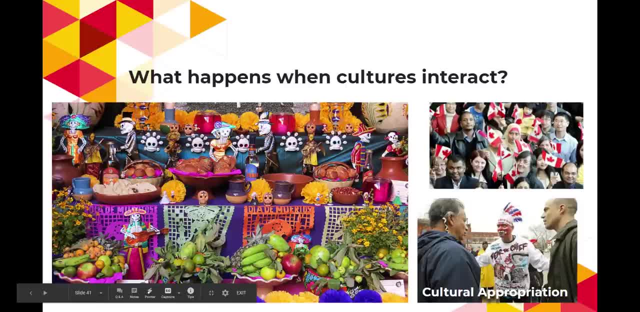 leave a comment if you would like. i try. leave a comment if you would like. i try to get back to as many of those as i can. to get back to as many of those as i can. to get back to as many of those as i can. good luck on whether it's your midterm. 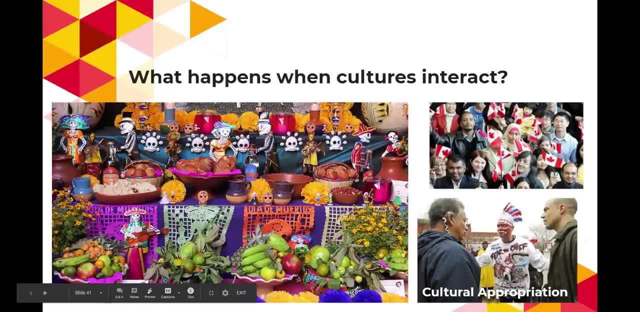 good luck on whether it's your midterm. good luck on whether it's your midterm or the national exam. best of luck to you or the national exam. best of luck to you or the national exam. best of luck to you, um, and i'll see you in the next one. bye. 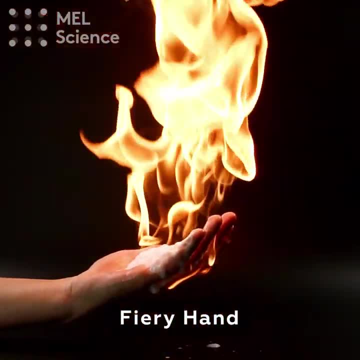 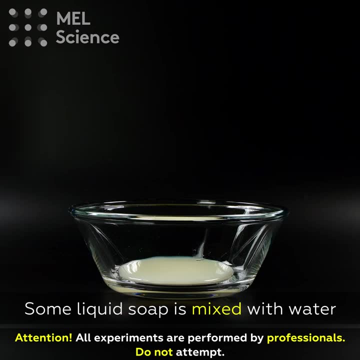 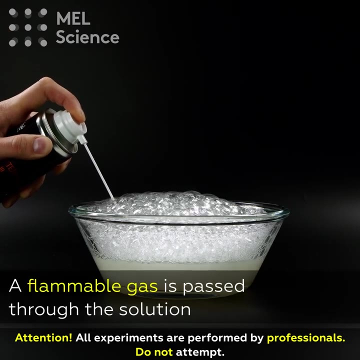 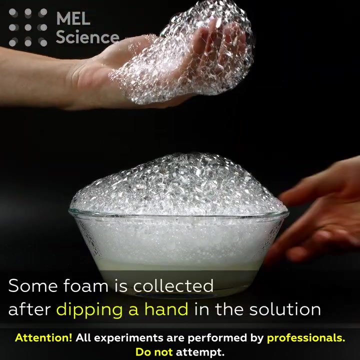 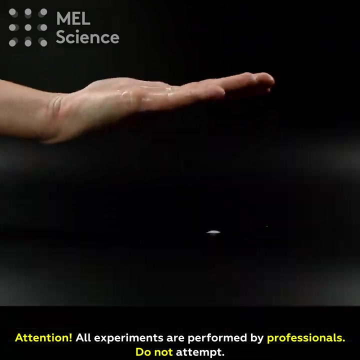 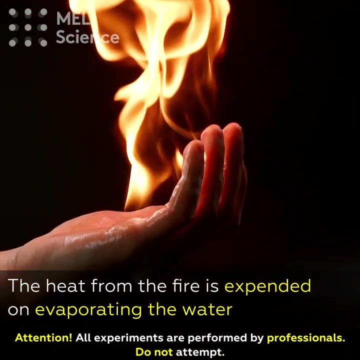 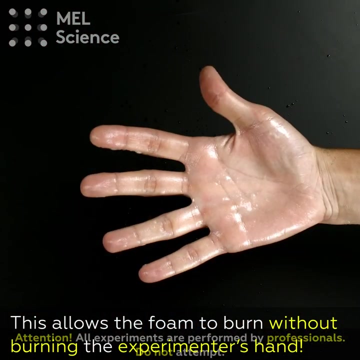 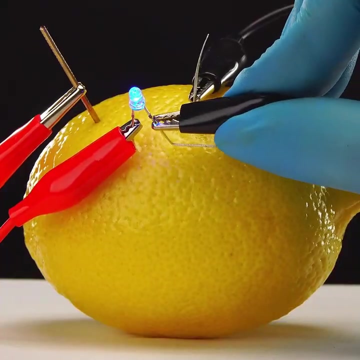 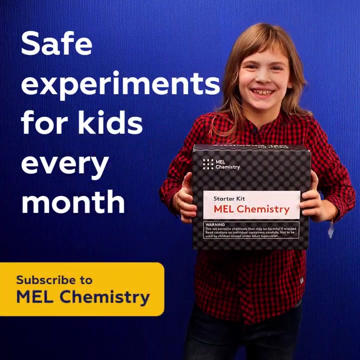 If you have any questions or other problems, please post them in the comments section of the video. If you have any questions or other problems, please post them in the appropriate places. Thank you for watching.